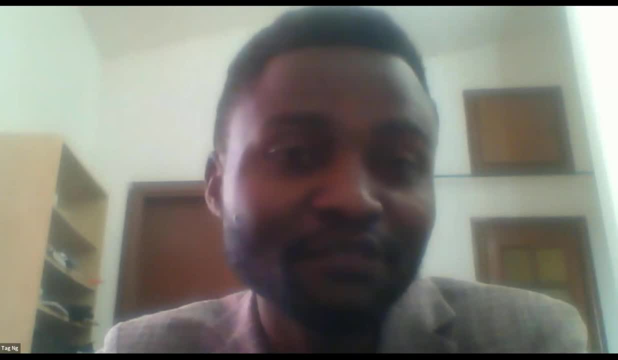 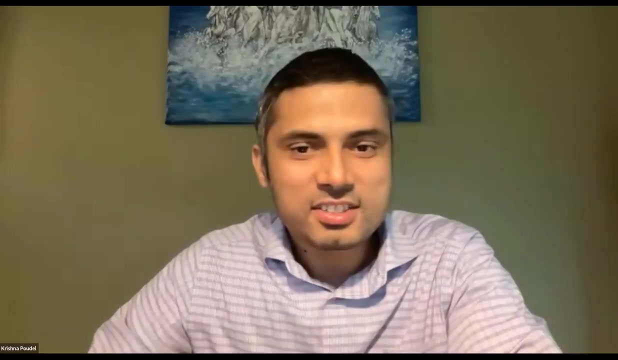 he has collaborated with Achivas Gadwin, one of the popular organizations in Africa poised at impacting the lives of young people. So, without wasting much of our time, I would love to welcome Professor Krishna Podia for his presentation. Thank you, All right. Thank you, Joshua, for that great introduction. 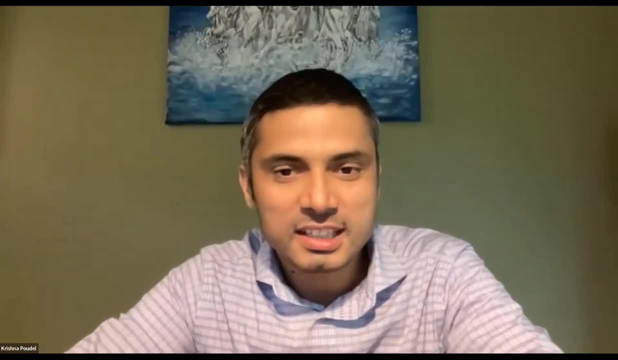 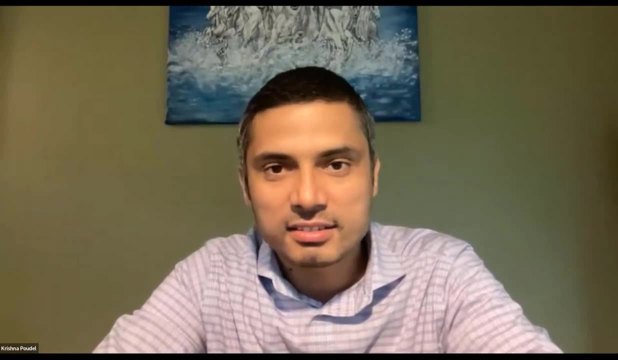 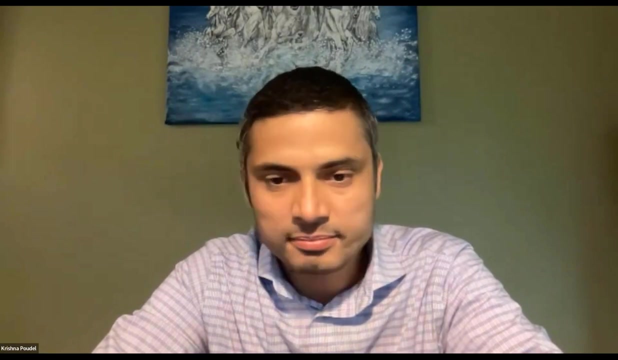 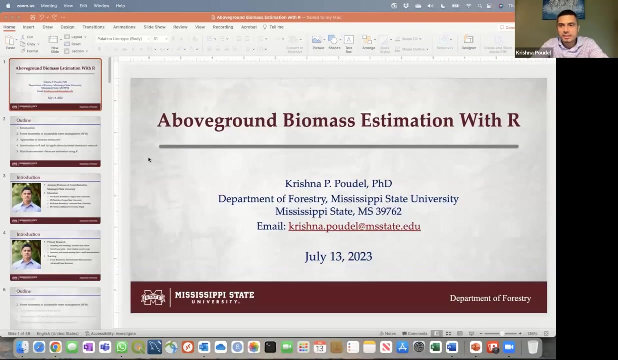 And thanks for the invitation to talk about above ground biomass estimation with R today. Hopefully, something that we will discuss Today will be useful for many of us. Let me share my screen, if I can. Can you see my screen? Yes, Okay, good. 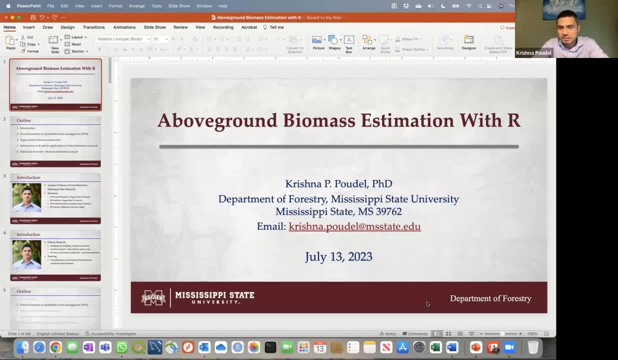 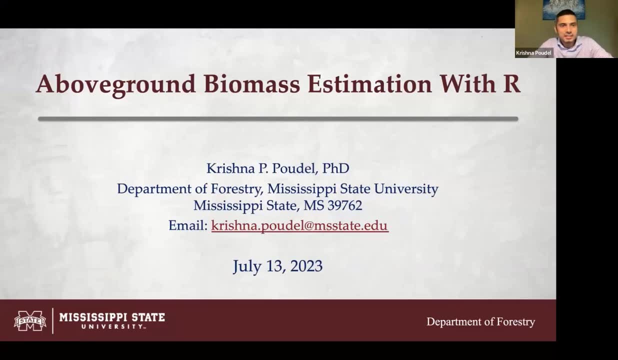 All right, I guess I can minimize that And let's make it full screen, All right. Thanks again, Joshua And everyone for joining. My name is Krishna Podia And I'm an assistant professor of forest biometrics here at Mississippi State University. 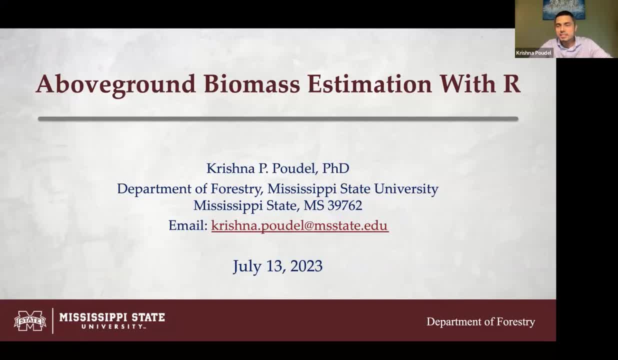 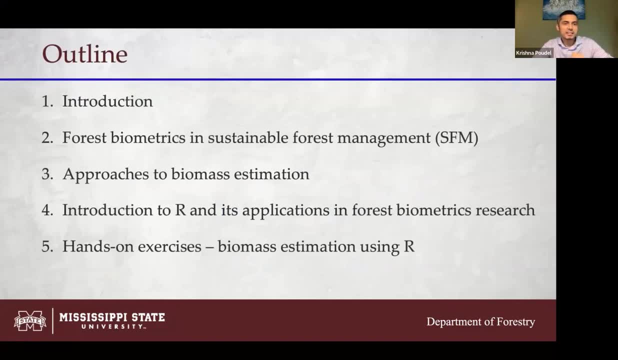 Today we'll talk about above ground biomass estimation with R. So this is the outline. I'll provide a brief introduction about myself and my research, And then we'll talk about forest biometrics in sustainable forest management- How biometrics can help us in sustainable forest management. 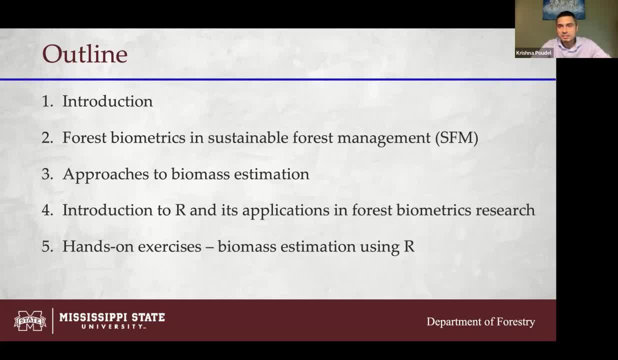 And then we'll talk about what are the common approaches that we use in biomass estimation. Then briefly about: I think I have a couple slides about introduction to R and its application in forest biometrics research And then later I will do some hands-on example for estimating biomass using R. 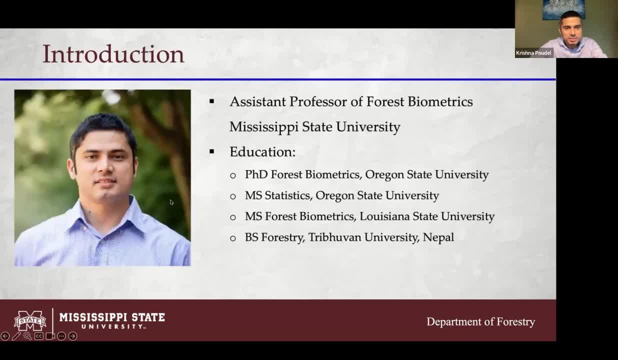 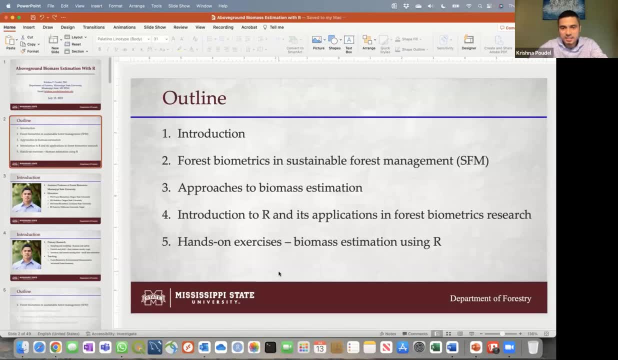 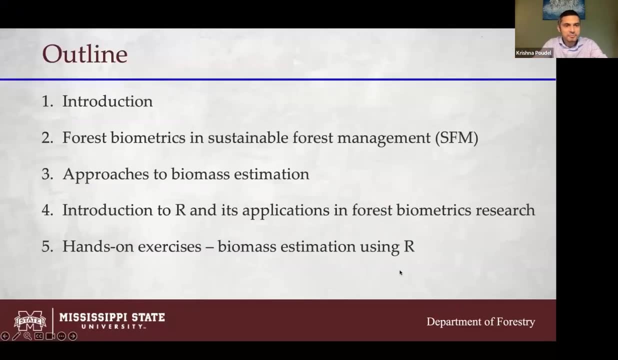 I have. I did post the link to data and R code on chat, But I think that got lost because we had to restart the machine, So I'll post that again later when we get to that point. Okay, So brief introduction. Like Joshua mentioned, I'm an assistant professor of forest biometrics. 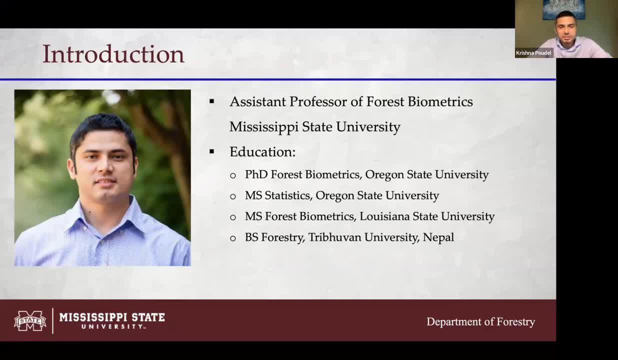 I started this position in 2018.. Before doing that, before starting or before coming here, I was a postdoc scholar at Oregon State University And I got my PhD in forest biometrics and master's in astronomy. I have a master's in statistics from Oregon State University. 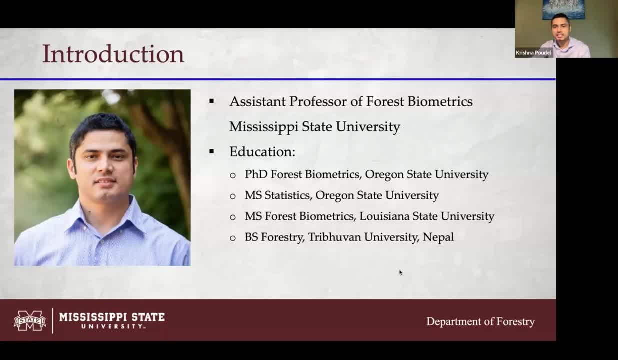 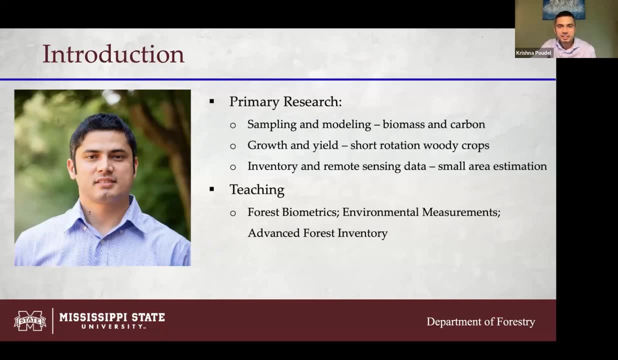 My master's in forest biometrics from Louisiana State University And my bachelor's in forestry from 311 University, Nepal, where I am originally from, And my primary research focuses on sampling and modeling. Recently, or in the last few years, I've been focusing on sampling and modeling for biomass and carbon estimation. 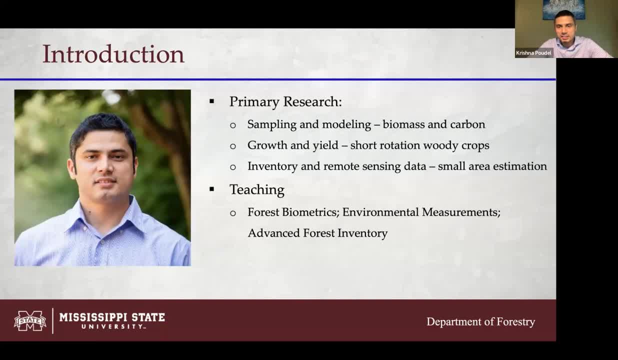 I have also worked with the growth and yield models and currently working on some soil tradition bioenergy crops and developing growth and yield models for them. I also work with forest inventory data and fusing or combining that with the remote sensing data. For example, it's malaria estimation. 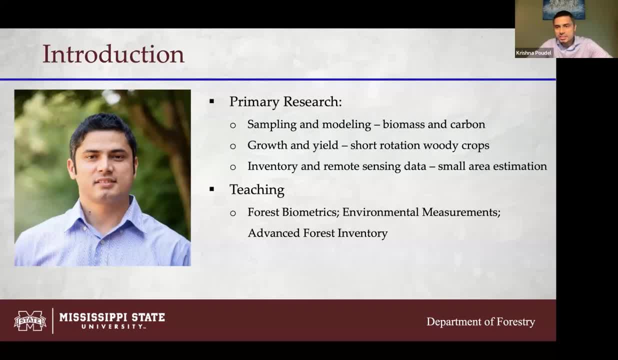 So basically fusing multisource data for a forest inventory problem. And in terms of teaching, I teach mainly three courses: forest biometrics, which is taught for both graduate and undergraduate students in our department. Environmental measurement, which is sampling design, which focuses on sampling design. 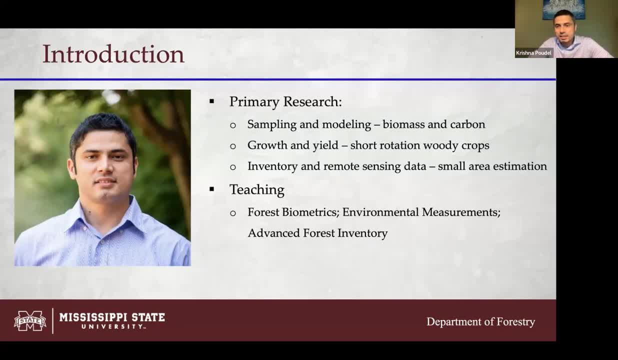 And that's designed for our natural resource environment conservation program students And advanced forest inventory, which is a graduate level course in forest inventory. We talk about regression analysis, Growth and yield models, Application of different regression models, Starting with a simple basic linear regression model to more complex models. 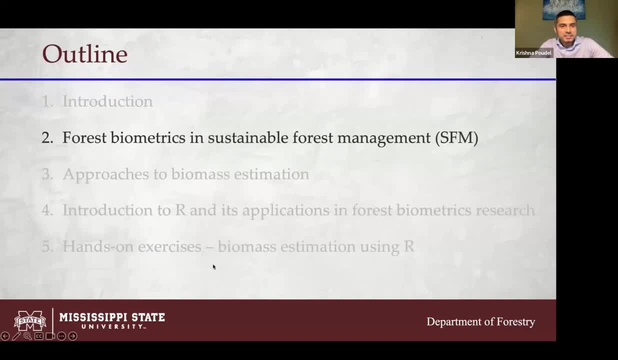 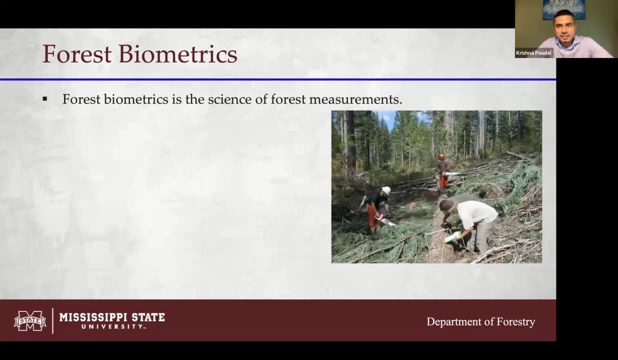 So that is my background information. Now let's talk about what forest biometrics is and how it is useful for sustainable forest management. I think you guys had some speakers before saying hi. I think he talked about what is forest biometrics as well. 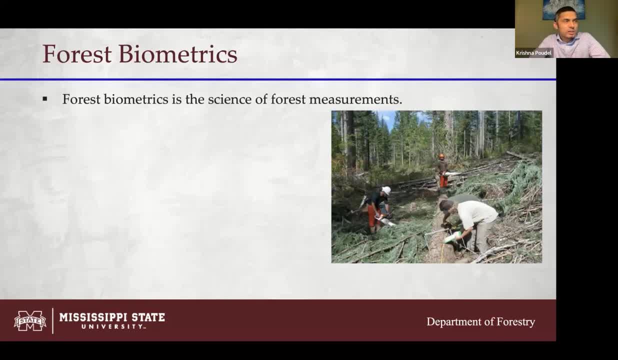 And I don't think there is one standard definition for forest biometrics, But it is a science of forest measurement. So what it does is it deals with the application of mathematical statistics So that we can use it to analyze the characteristics or features of trees and stand. 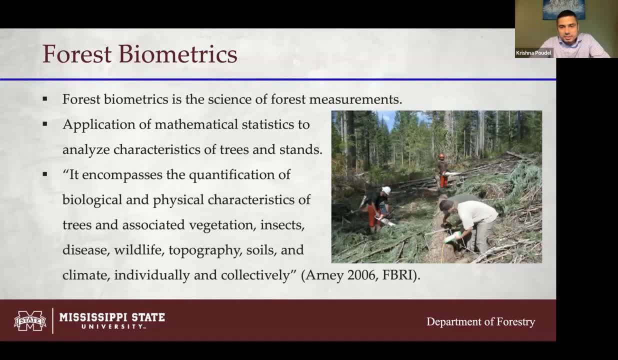 And Arne 2006.. From forest biometrics research institute, He provided more comprehensive definition for forest biometrics, Which is? it encompasses the quantification of biological and physical characteristics of trees and associated vegetation, insect disease, wildlife, topography- So many things. 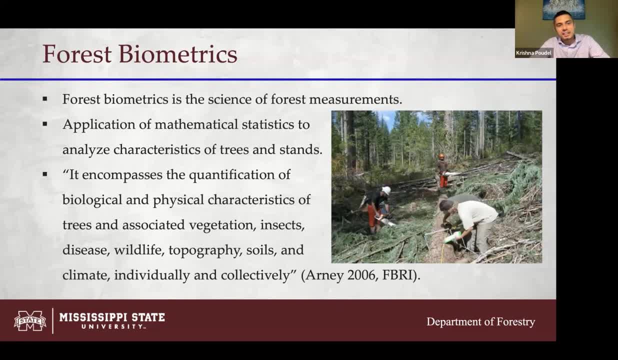 So we are focused on trees, But how they are associated with other aspects of the environment. So biometrics is. it has two components: Biological and measurement. So it's a biological measurement, But we are focused on biometric forest measurement of forest. 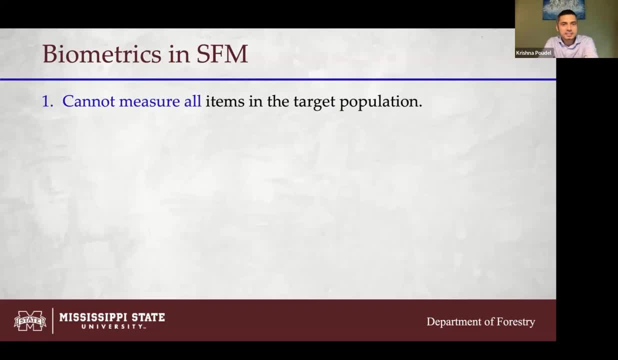 So how can biometrics help in sustainable forest management? So if we want to manage our resources sustainably, Then we need to know or we need to have the up-to-date information or up-to-date inventory of our resources. However, because the forest resources are spread across the large area, 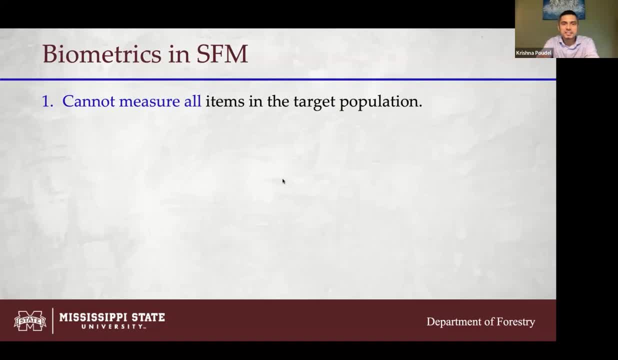 So we cannot measure all the items in our target population. That's one of the main challenges we have. And biometrics. through biometrics we can learn about different sampling designs Which help us in getting the unbiased estimate of our variable of interest. 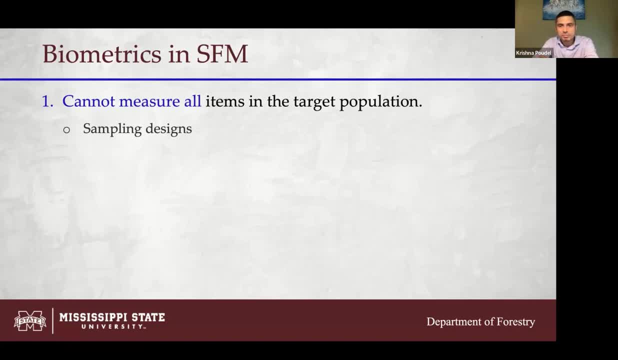 For example, are we interested in volume per hectare or per acre, Or are we interested in carbon sequestered by a forest? So those kind of things We can use. sampling designs- I think Dr Matt Russell talked about sampling designs applicable in natural resource management. 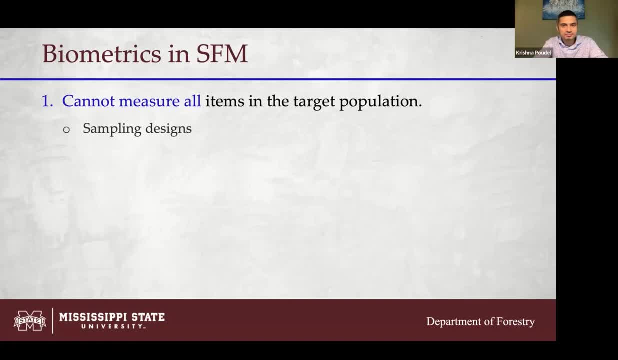 So for those of you who joined the previous seminar. And the second problem in resource inventory is we cannot. even when we sample, Then we cannot measure some of the variable of our interest. If we take a simple example of height and diameter measurement for trees, 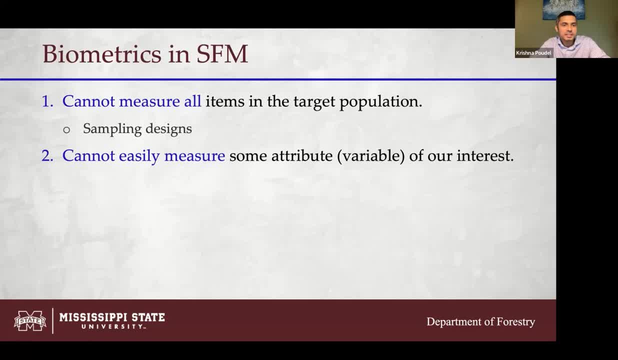 Diameter it's easy to measure, But height it is difficult to measure. So in that case what we can do is measure diameter and height for sample trees And then develop regression models, Which we learn in biometrics as well. And the third problem is we are not just interested in what is out there for us. 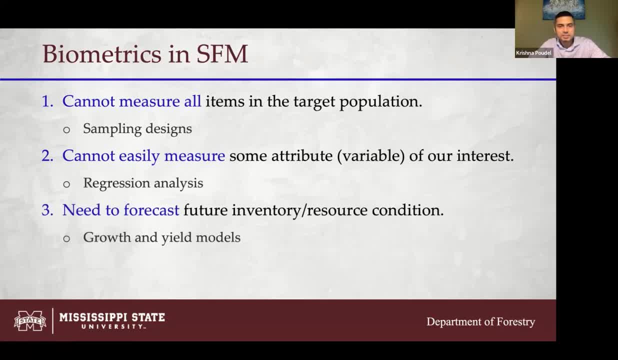 We are not just interested in what is out there right now, But we also want to know what the forest or the resource condition will be in the future. So for that reason we need growth and yield models, Which are also tools developed using biometrics research. 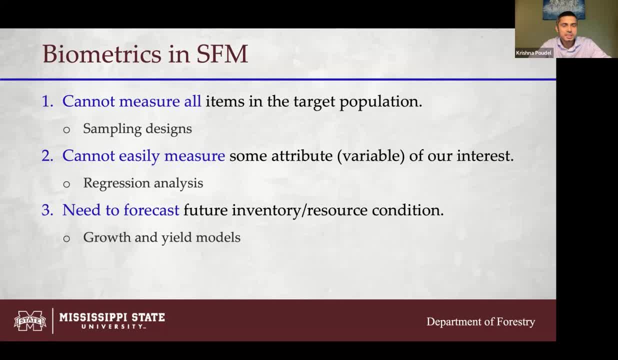 So basically, three main problems in managing our resources sustainably: Because we want to get the up-to-date information But cannot measure all items, Cannot easily measure some And we need to know what the standard, what the forest will look like in the future. 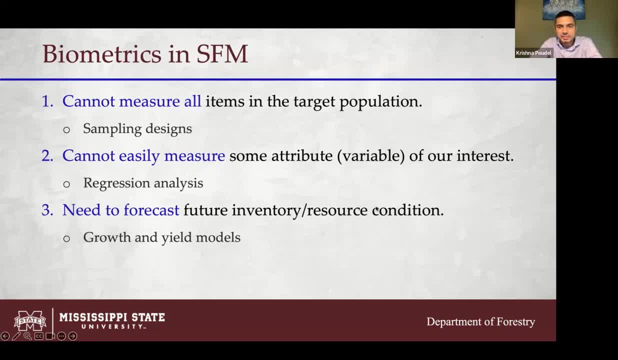 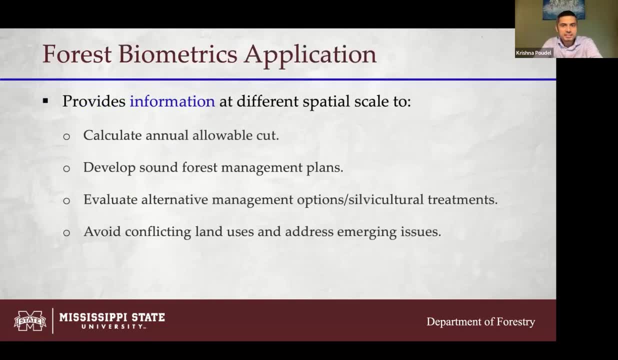 And biometrics. knowledge of forest biometrics can help us solve those problems. And then, so to summarize, So how does forest biometrics solve that problem? It provides information at different spatial scale So that we can calculate what is the allowable cut. 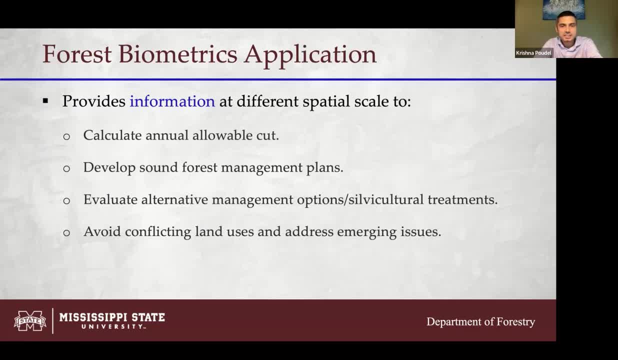 How much volume we can get out of that And how much we have to stand on a sustainable basis. And that helps us in developing some forest management plan And we can also use that information for evaluating different management options And what are some silvicultural treatments we need to apply for our to meet our target objective. 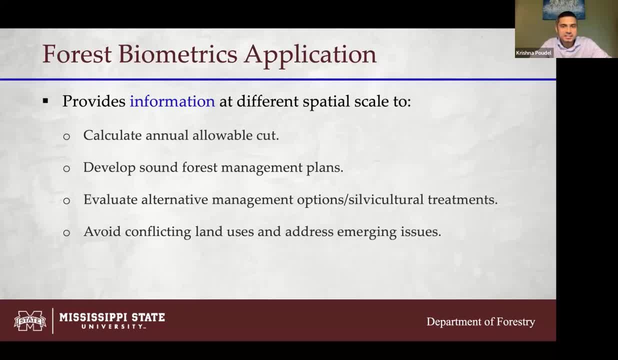 For example, do we need to do some kind of peening? Is the stand ready for harvest? Those kind of things? We need some quantitative measure And forest biometrics helps us in that And it also helps us in avoiding conflicting land uses. 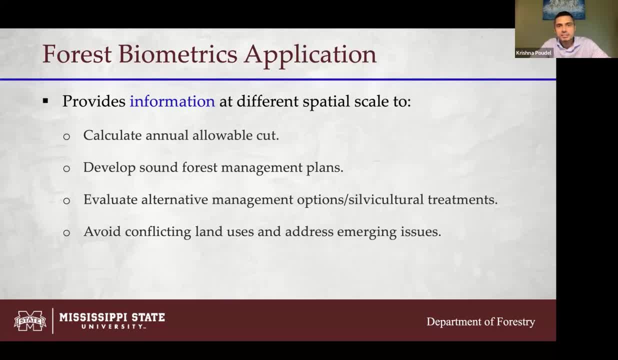 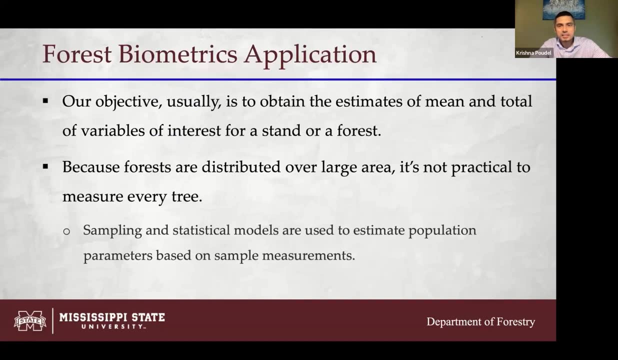 Addressing emerging issues, For example carbon sequestration. That issue is also: we need forest biometrics to be able to quantify forest carbon sequestration as well. So basically our objective usually in forest measurement is: we want to know the mean or total of the variable of interest. 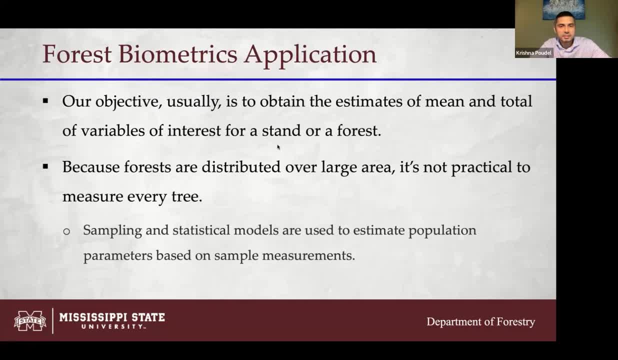 For example volume per acre or hectare Or carbon per hectare. But because the forests are distributed over large area So we cannot actually measure all the trees. So that means we use sampling and statistical models Through forest biometrics And then use sample based estimate as the 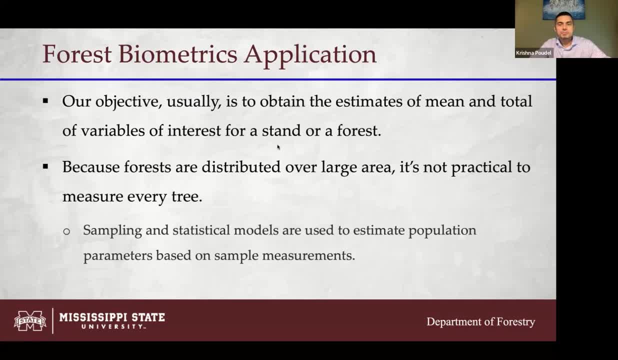 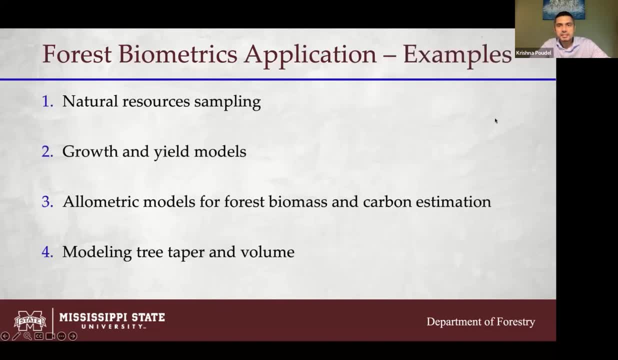 as the guiding attributes for decision making. So these are some of the examples of forest biometrics application that I have used in my research. First, the natural resource sampling, For example, what is the appropriate or what is the best method to sample for estimating forest carbon? 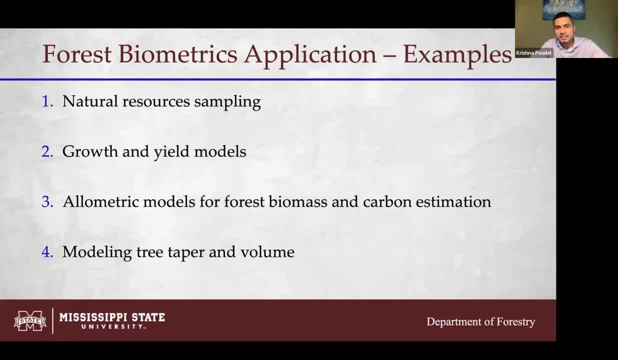 And growth and yield models. What do they stand will look like? I have looked at multiple different types of growth and yield models, For example, whole stand model, Stand table, projection, diameter, distribution models, If you guys are familiar with those. 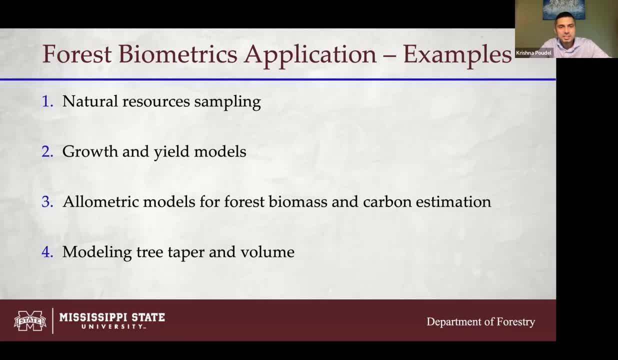 And also elementary model development for biomass and carbon estimation. This is critical And that's the main focus of today's talk- And modeling tree taper and volume. So, for example, depending on what is the merchandising diameter limit, we need to know what is the upper estim diameter. 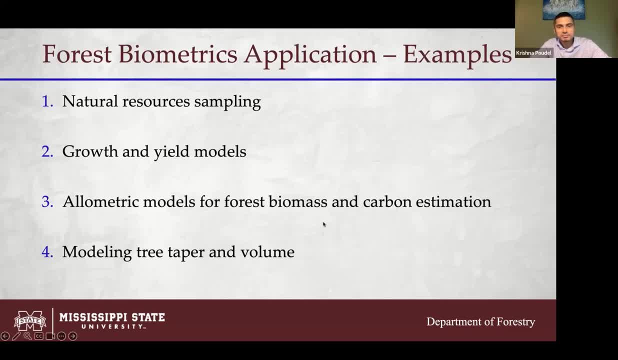 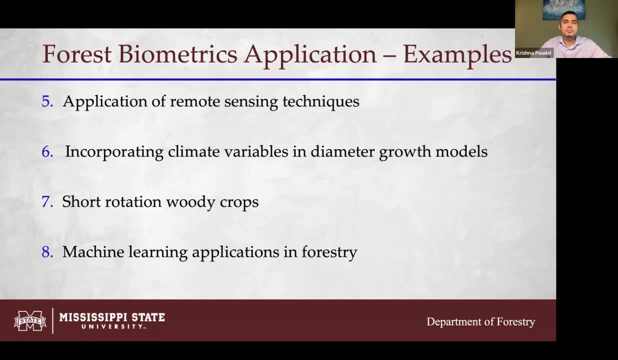 So for that we need tree taper and volume equations, And biometrics is one application of forest biometrics. research is in that area. Similarly, remote sensing technique. We use different types of remote sensing data for answering our problem or natural resource management questions. 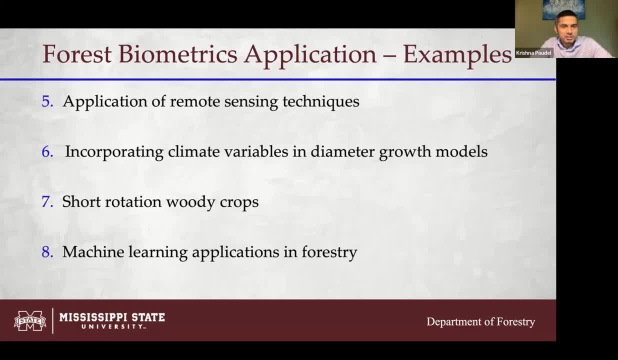 And also incorporating climate variables in our growth and yield models. Because of the changing climate, we can expect different growth pattern in our forest, So we need to incorporate that And biometrics is one application of biometrics in that area And soil protection. woody crops. 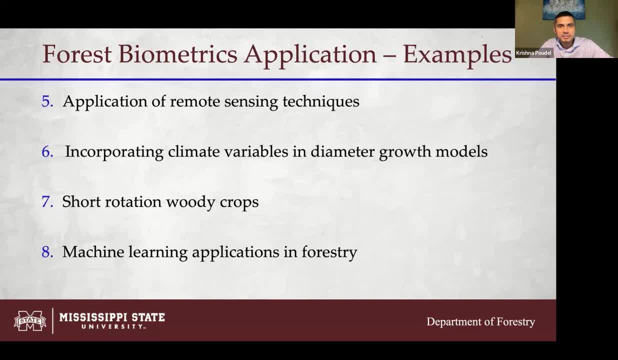 These are the biodegraded bioenergy crops that are planted for producing biofuel, And if we want to identify how much feed is stuck, how much this plantation can supply, then we need to understand the growth and yield of these type of crops as well. 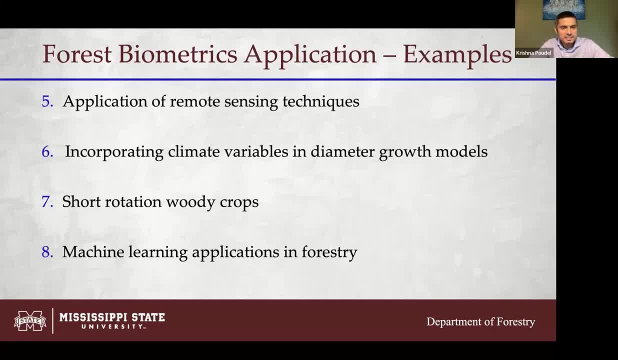 And also very popular these days: machine learning in forestry, Different types of artificial neural network and different methods Those are used in forest as biometrics tool in different forestry applications. So these are basically some of the research projects that I have worked on. 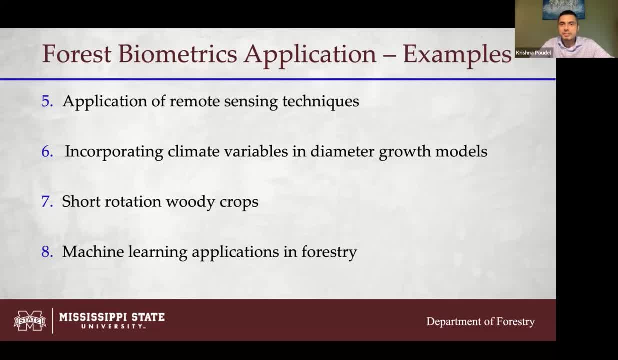 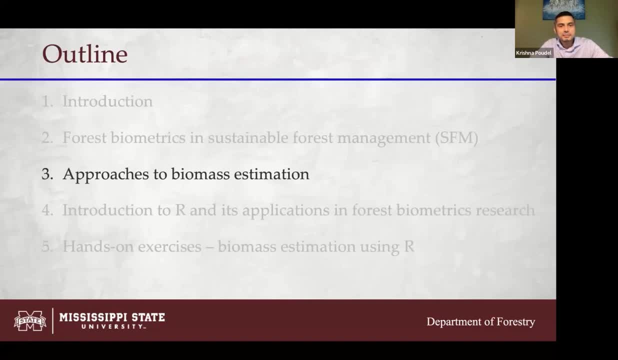 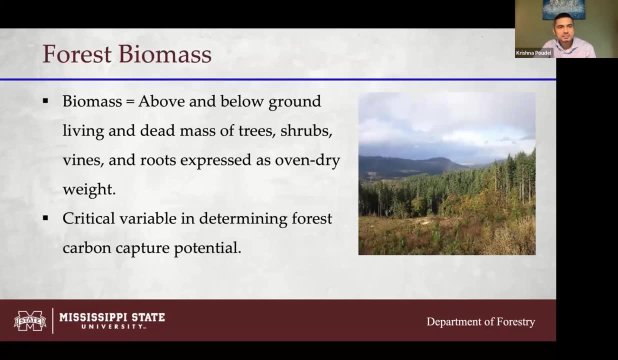 And these are related to the forest biometrics. Okay, so now let's move forward with the approaches to estimate biomass, And we'll focus on above ground biomass today. So first let's define the biomass. So it is above and below ground living and dead mass of the trees, shrubs, vines and roots. 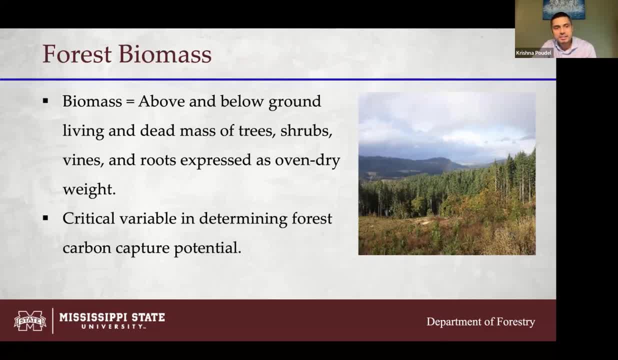 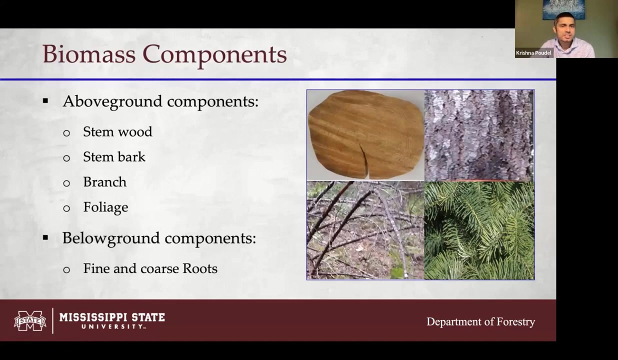 And we usually express this as open dry weight. And why do we care about forest biomass? Because it is the critical variable in determining what is, or how much carbon is, our forest capturing. So for that reason we have to estimate biomass And we can divide this biomass into two, or forest biomass or tree biomass, into two different components. 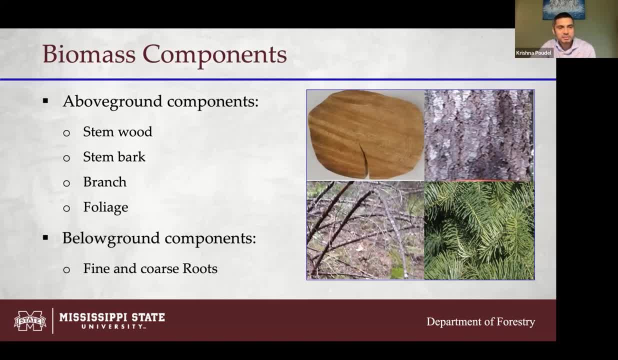 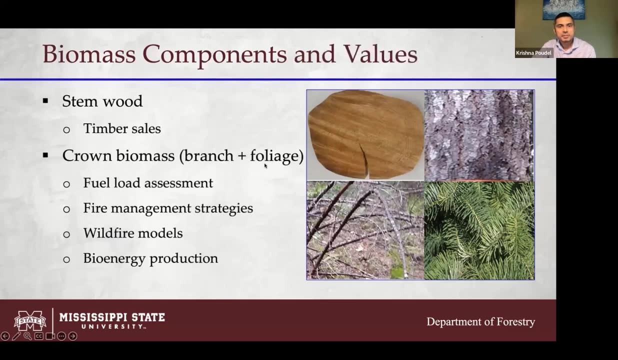 Above ground biomass and below ground biomass component. Above ground for the tree it would include stem, wood biomass, stem, bark, branch and foliage or leaf. And for the below ground component we have fine and coarse roots. And why do we care about the components is because they have different values. 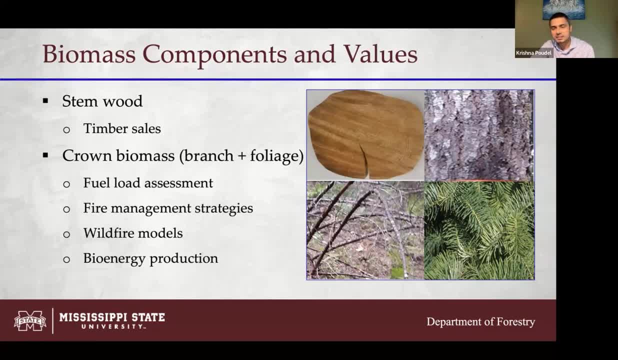 For example, stem wood biomass is used for information about the stem wood. biomass is used for timber sales, Crown biomass including foliage and branch. it provides information for fuel load assessment. It can be used to develop our fire management strategies, Depending on how much biomass is left over after harvesting. 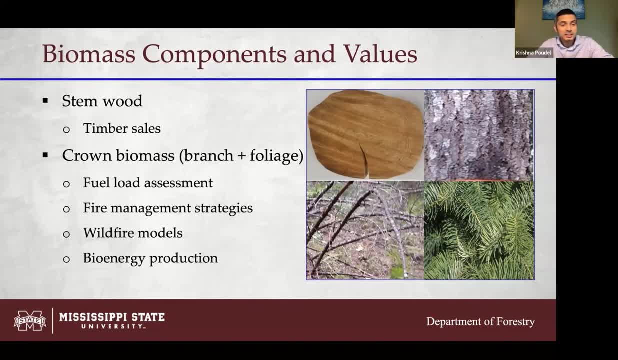 we can decide how much fuel is in there, or we can determine that, And that can be input in our wildfire models. And also, if we want to use these leftover material for bioenergy production, then we need to know what is, or how much is, there. 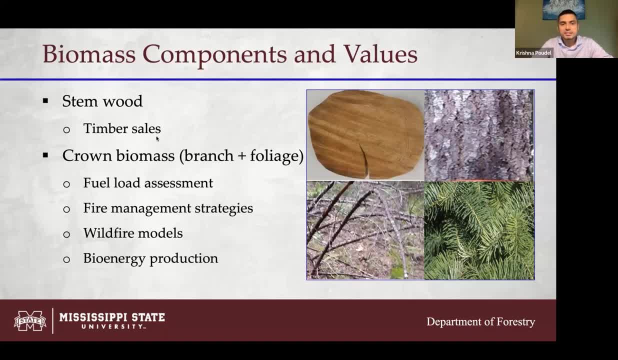 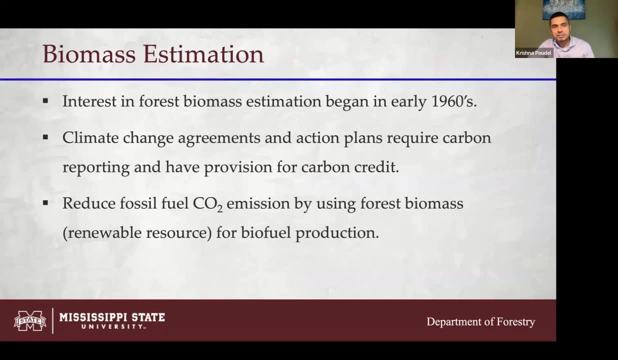 And that's why we use the carbon biomass in the ground component. So that's why, instead of just in addition to the total above ground and below ground biomass, we are also interested in different component biomass And estimating biomass. it's not new. 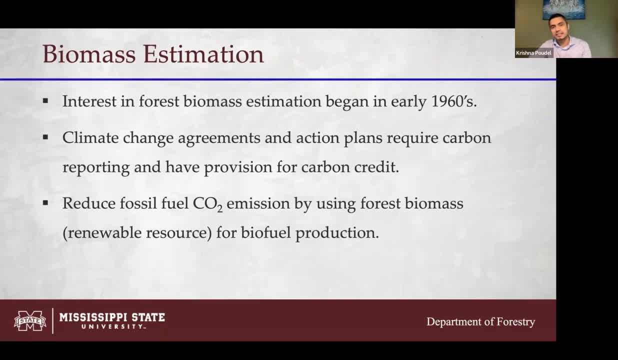 The interest started, or began, in the early 1960s, And these days, because of different climate change agreements and action plan, we have to estimate carbon And instead of estimating carbon directly, we estimate biomass and then convert that into carbon estimate. 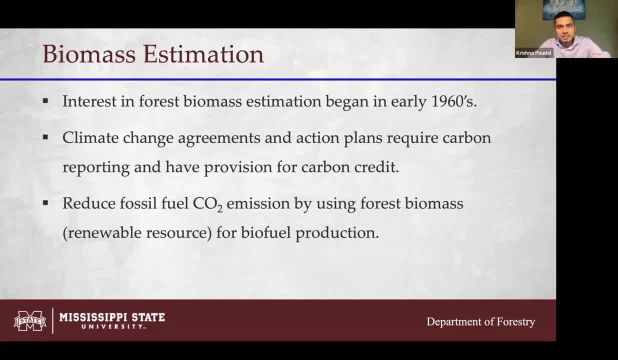 And, for example, REDD+. they have the provision for carbon credit By depending on how much carbon your forests are sequestering, then you get credit for that. So for that reason also we need to. there has been an increase in interest in estimating biomass. 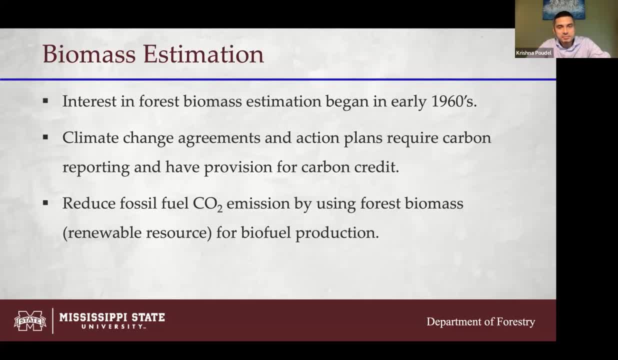 Also, if we want to reduce fossil fuel emission by using biomass as the renewable source of energy, then we need to know how much biomass is available for biofuel production, And that information is also useful for establishing where we should locate our bioenergy plants. 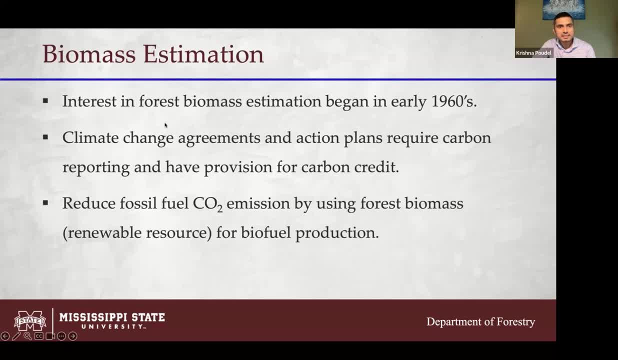 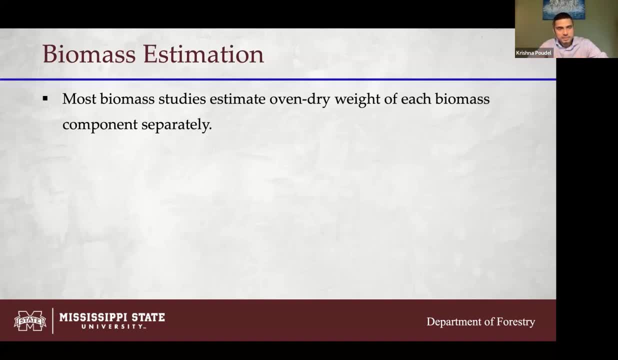 So, for that reason also, we need biomass estimate. And so now? so there is two parts: One is biomass estimation and the other is biomass measurement. So biomass measurement would be actual measurement. Estimation would be based on some models or sampling. 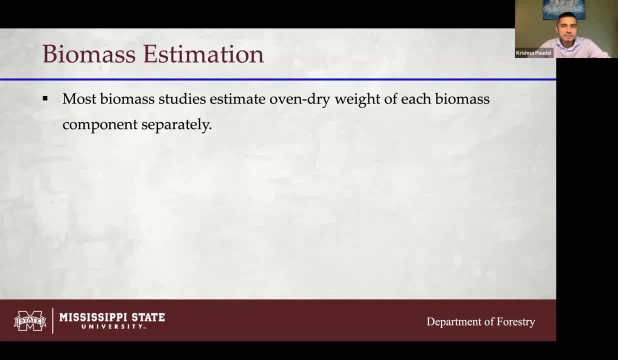 So most biomass studies. they use open dry biomass or open dry weight and calculate the biomass of different components separately. And this is for measurement. If we have young trees then it is measured. It is measured usually by fitting the sample tree and weighing the entire tree. 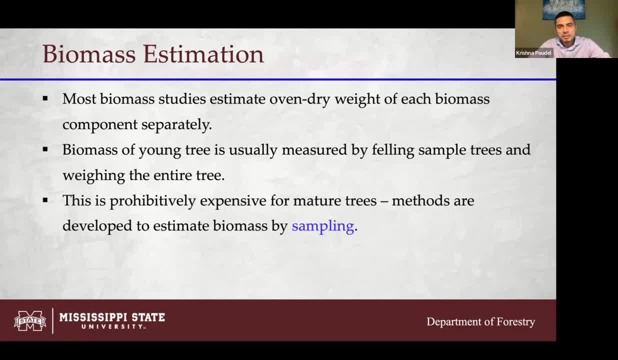 So this is for measurement, And, but it is prohibitively expensive. It is difficult for mature trees because they are large, So it takes, it will be labor intensive and it will be costly as well. So instead of measuring the entire tree, 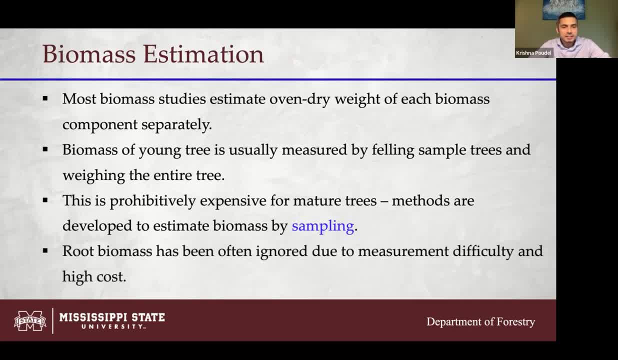 we use some kind of sampling And root biomass. before starting this talk, I talked with Joshua about the below ground biomass as well, And there is comparatively there has been fewer research focused on below ground biomass because it is difficult and also costly. 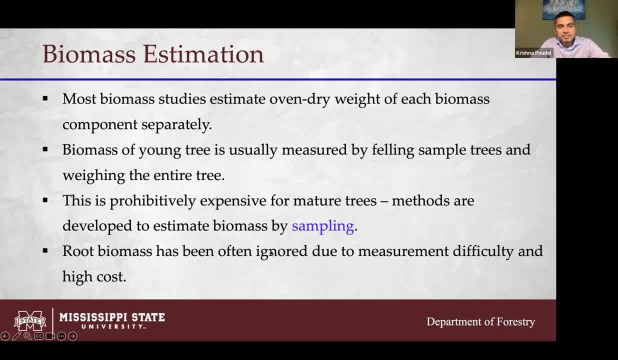 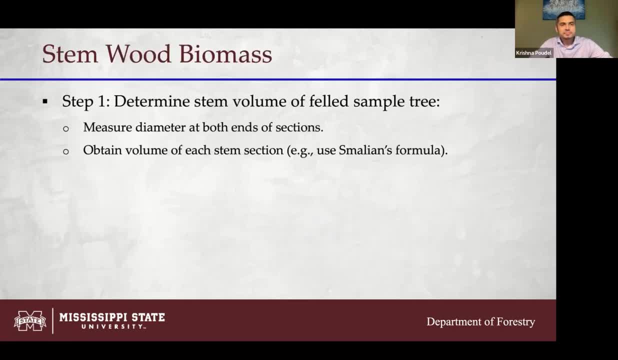 So that's why it's been- I don't know, ignored is the right word, but it has not been done as much, And so how do we measure biomass? So let's first focus on how do we measure biomass, Because when we want to estimate, 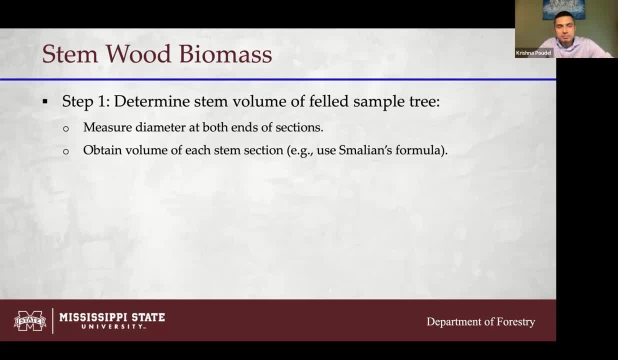 then we need the some measured values, or Y values, for our regression model, And how do we get that? So, so the first step is to collect data. that, let's say, if we want to measure the steam wood biomass, then how do we do that for mature trees is determine steam volume. 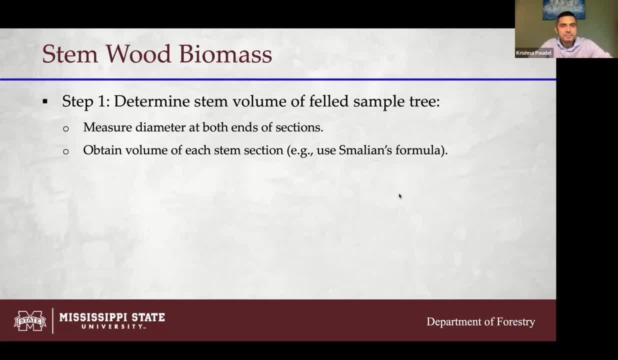 by sampling or destructively sampling some trees, And we measure. once we harvest the tree, then we measure diameter. we section those logs and then measure the diameter at both ends. And we can use volume calculation formulas, for example Smedian's formula. 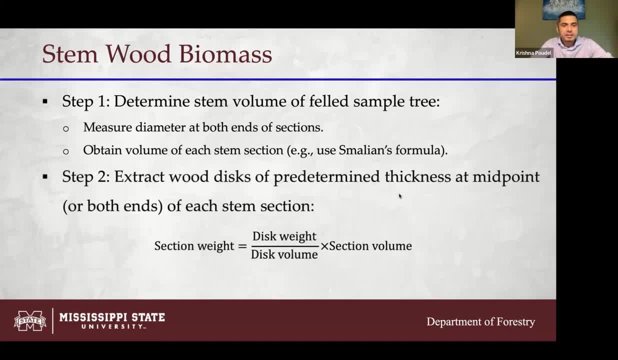 and obtain the volume of each section. Then we also get some disk, sample disk of predetermined thickness. It can be at the midpoint or midpoint of the section or from both ends of the section. And then, once we get that, then we use the ratio of disk weight to disk volume. 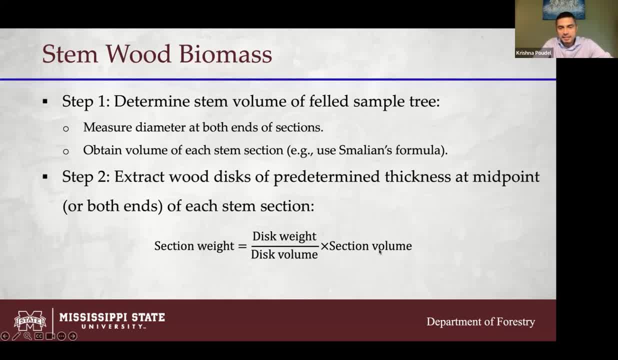 like here, and then multiply that by the section volume, which we calculate using Smedian's formula, So that would give us the section weight. And once we get the section weight for all the sections, then we can add them together to get the 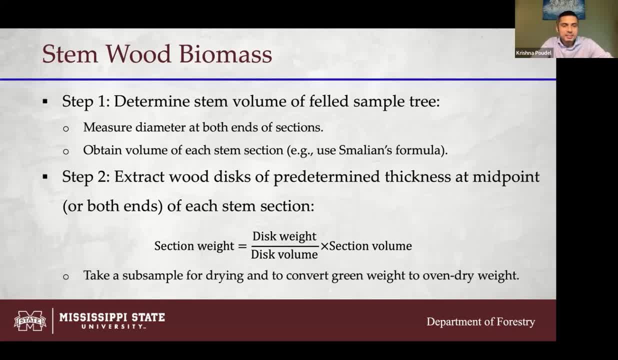 total steam wood, biomass or green weight. And then we also get the subset weight sample from disk so that we can get the ratio of green to dry weight which we can apply to convert that section green weight into section dry weight or total green weight to total steam wood dry weight. 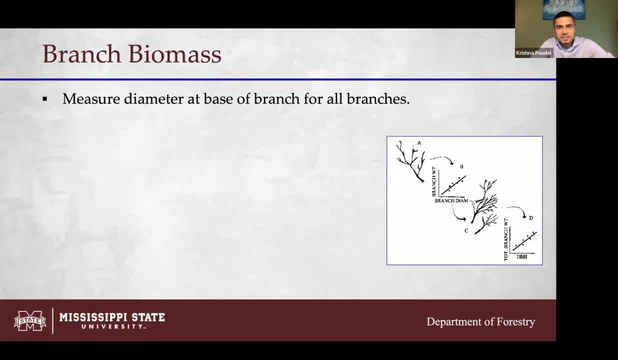 And for the branch it is more challenging because there are too many branches. The idea is: first we measure diameter at the base of all branches, then take a random sample of branches and obtain their individual green weight or dry weight And then these observed branch weights. 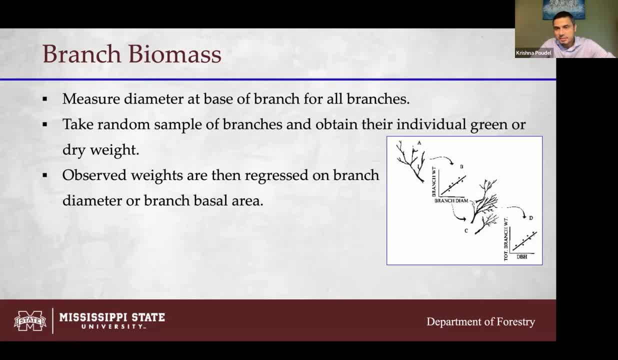 individual branch weights. they are regressed, or we fit regression model that predicts the individual branch weight based on branch diameter or branch basal area, And then once we calculate the individual, once we have the model for predicting individual branch weight, then we can use the diameter measure. 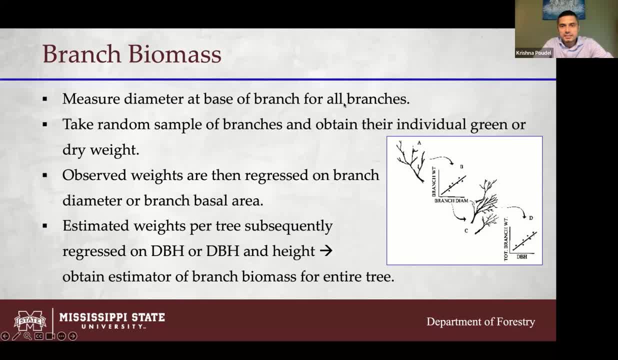 step one diameter of all the branches and apply that regression model to get the green weight or dry weight of all the branches. And once you have the estimated dry or green weight of all the branches we add them together to get the total tree level branch biomass. 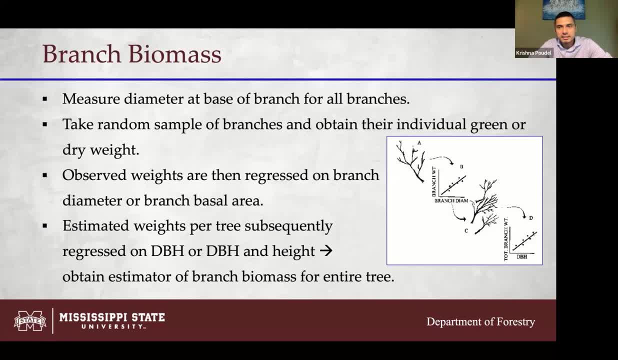 And then at the end we relate that tree level, branch biomass, not the individual branch level but individual tree level, with the diameter at breast height and other variables, For example total tree height- Sometimes we use height to the base of light ground. 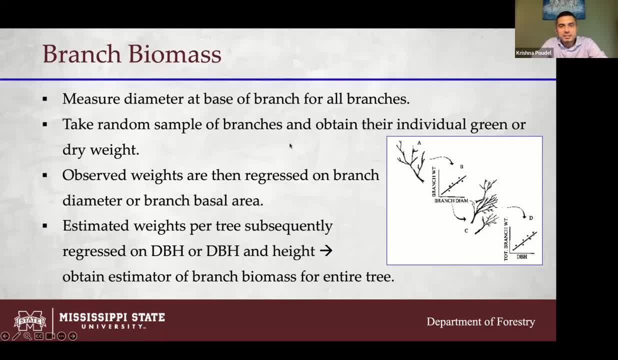 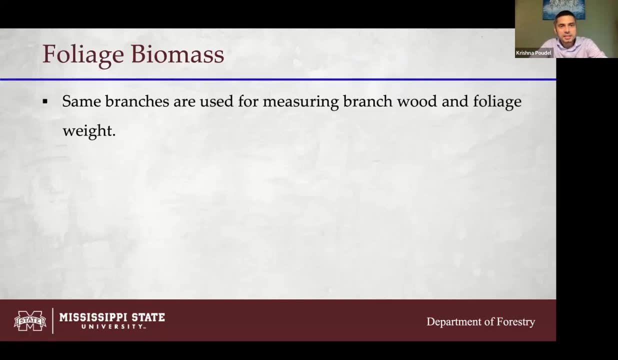 so that we can predict the total branch biomass for the individual tree instead of just the individual branch. Then for the foliage or the leaf we use the same branches that we measure for branch wood biomass And, for example, we can select a 25% random sample of branches. 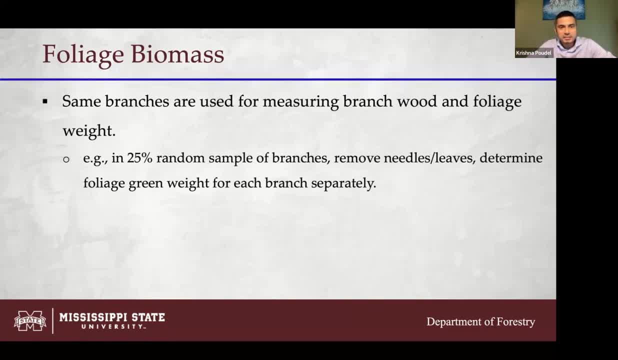 and get the foliage green weight for each branch separately and then fit same as in branch wood biomass. we fit regression model to estimate foliage biomass from branch diameter and then subsample for converting green foliage into open dry weight. And then, once you do that, 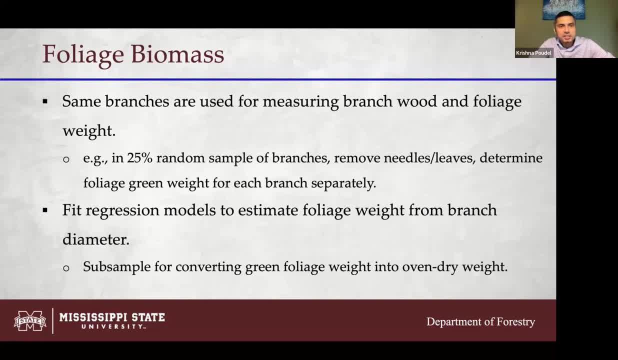 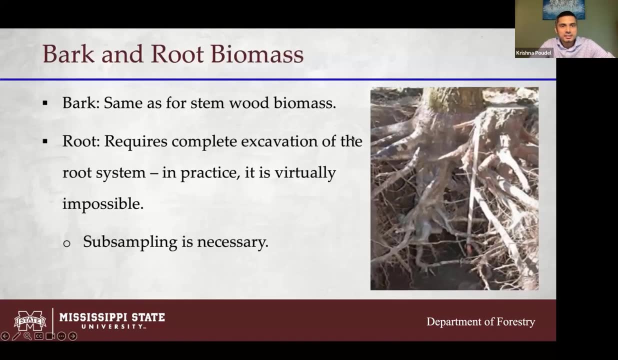 then at the end we add the individual tree foliage biomass to get the total tree foliage biomass and regress that with the tree diameter height to the crown base or total tree height. And the other components include bark and root biomass. Bark: 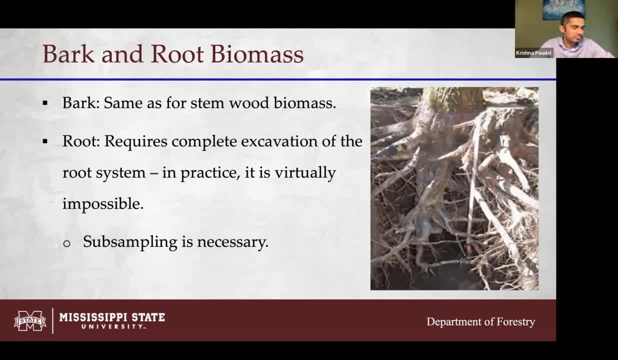 we do the same as in stem wood biomass, but instead of using diameter inside bark, now we use the diameter outside bark and we can calculate the difference between inside bark biomass and outside bark biomass and get the bark biomass For the root. 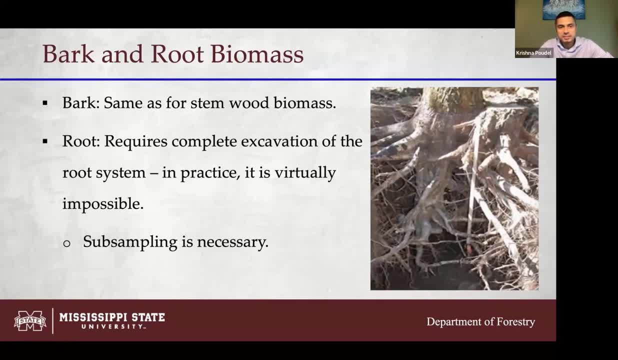 it is difficult. We need to excavate the entire root system, which is virtually impossible, so subsampling is necessary, And there is not enough. there is not large dataset for this, for the root biomass, And so this, this is. 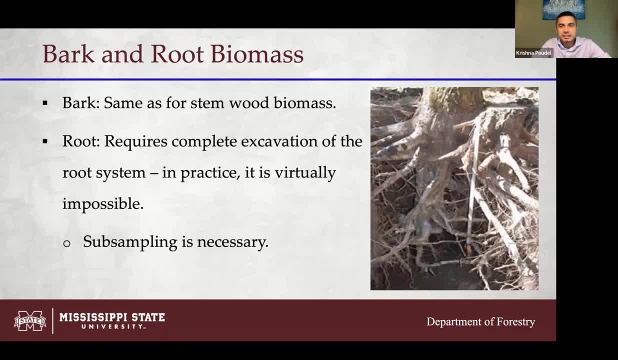 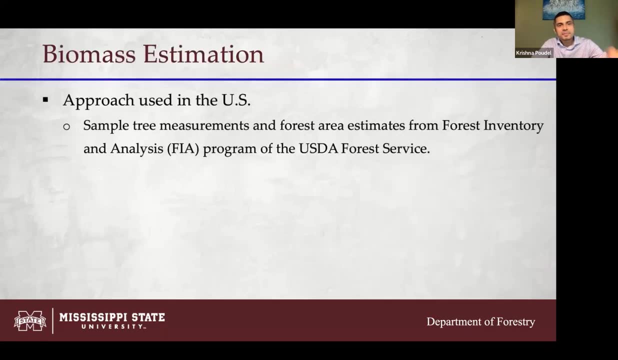 so far. what we talked about is biomass measurement. Okay, Of course we had regression model for individual branch biomass and foliage biomass, but this is also- that is also part of the measurement. Then the next is: next is we. 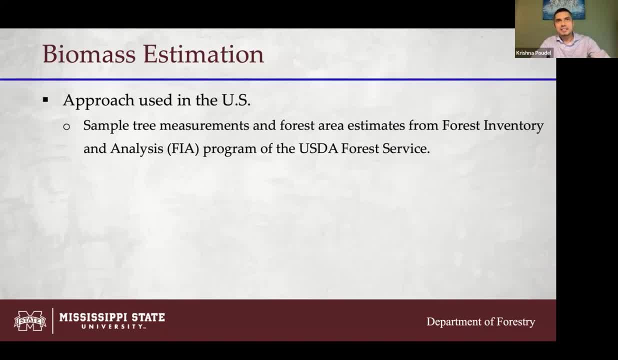 how do we estimate? So once we have the data for for developing model, so what we? how we estimate the biomass? So before starting that, let's talk about the biomass estimation approach used in the official greenhouse gas inventory. 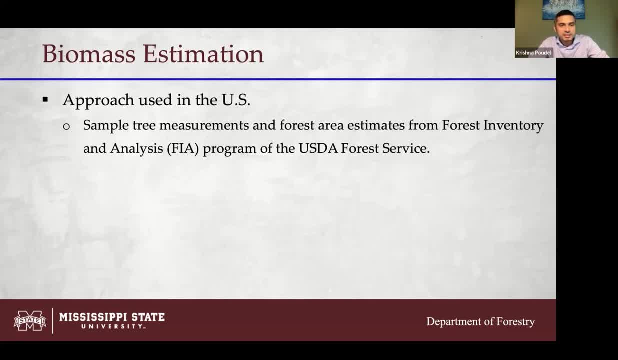 by the United States. In the US there is a forest inventory and analysis program which is part of the US, which is a program under US Department of Agriculture Forest Service And it is called the Census of the Forest. 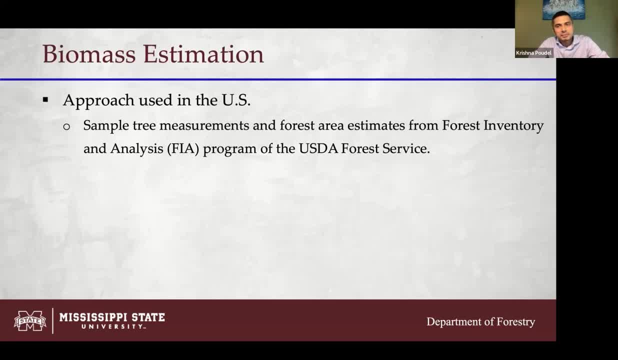 US Forest because they have permanent plots and those are repeatedly measured And that inventory data is used for used as the guideline or used as the main starting point for estimating forest carbon. So, tree measurement- once you have the tree measurement, 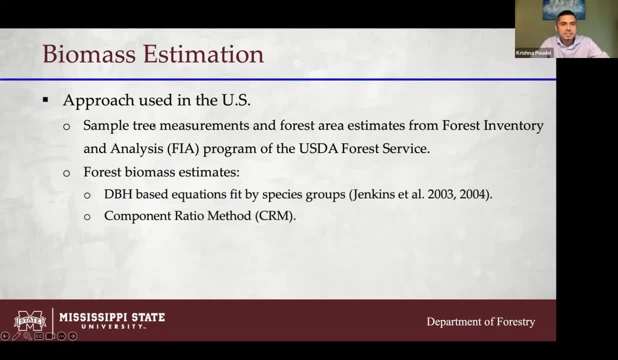 then we need biomass estimation for those trees. So in step one of this, in this case we have we have tree level information, for example diameter, height and other variables, tree level variables. And then, once we have that information, 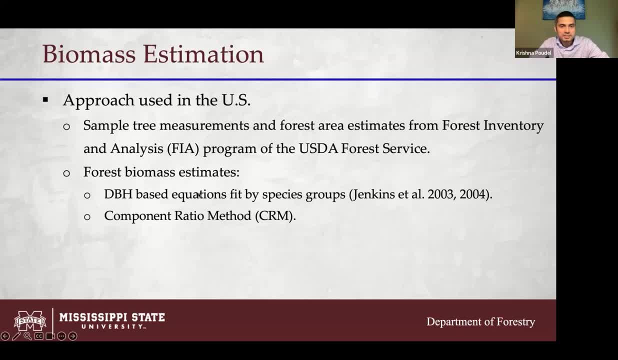 we we have different type of biomass equations that we can apply to those inventory data. Until 2009,, the US used to use DBS based or diameter based equations by species group, and those were developed by. 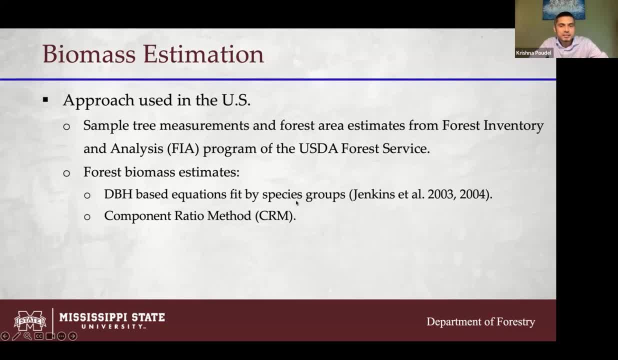 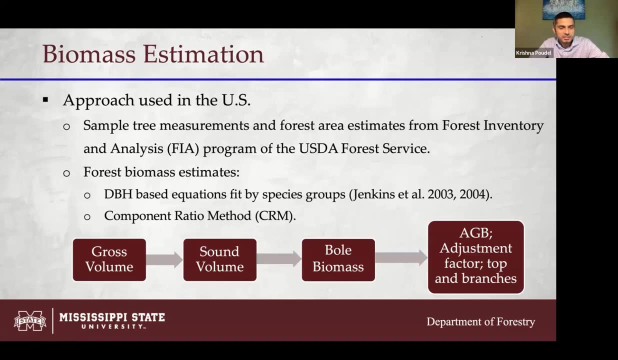 Jenkins and others in 2003 and four, And since 2009, the US. US is using a method called component ratio method. So basically the idea in component ratio method is: first use volume equation to get the gross volume. 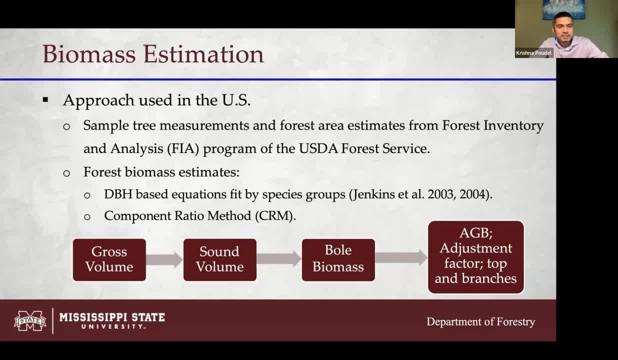 which is without accounting for defects, and then subtract that defect to get the sound volume And then convert that sound volume using wood density to get the bowl biomass And then, using some equations from Jenkins, then calculate some kind of adjustment factor. 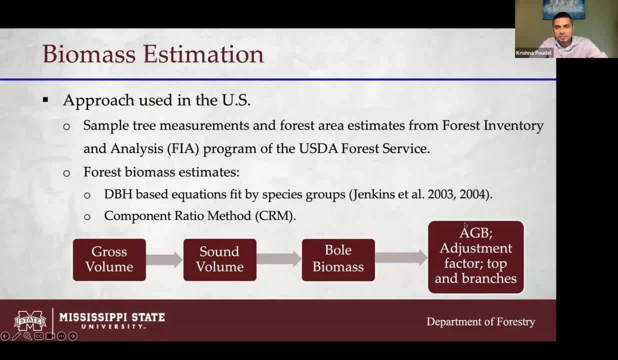 and then calculate other component biomass. So it's a kind of convoluted process. but it starts with the volume data, because there is a really large data set for tree volume And because historically volume estimation has been. 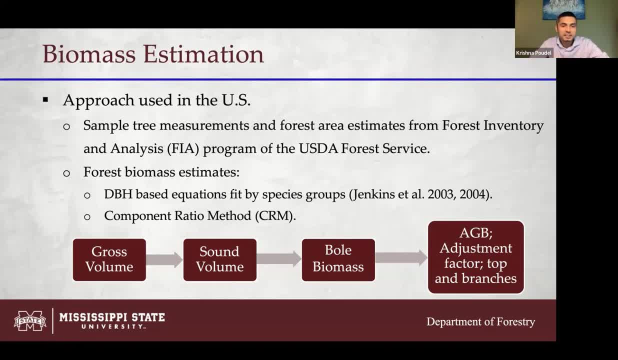 the focus. But biomass has not been. historically, it has not been studied as as much as volume. So that's why, to utilize that large volume data set, the estimation of biomass starts with the volume estimates. 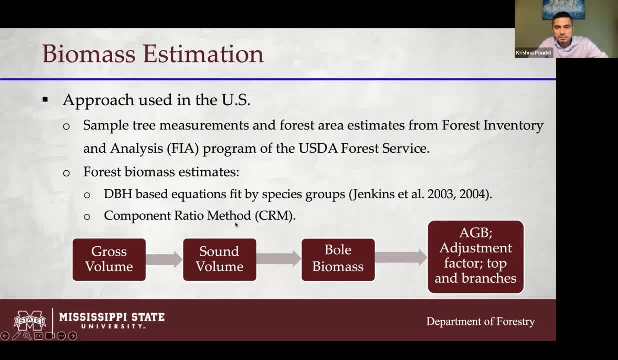 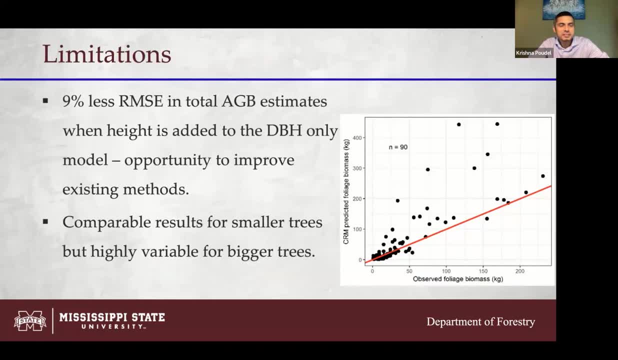 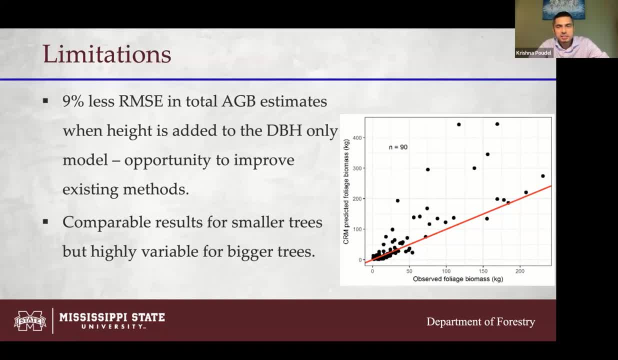 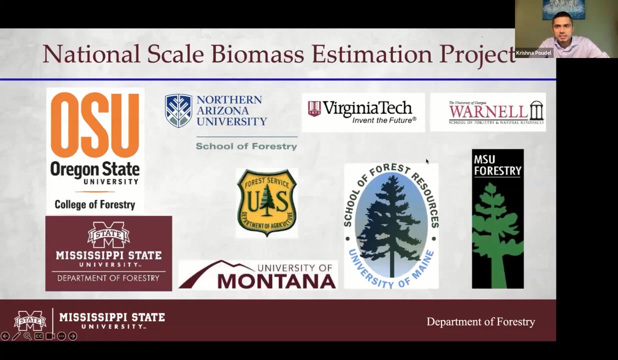 the, the, the These are, this is the Here, this is the, this, this data that I'm going to come in here and I'm going to directly check countries. the error was higher, So what we did is: in 2012, there was a nationally. 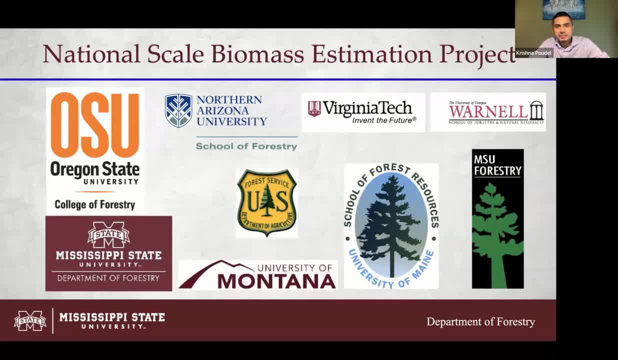 scaled effort to estimate biomass for the entire United States. There were seven different universities involved and it was led by the US Forest Service FIE program and Mississippi State University. So I was at Oregon State University so I started working on that. 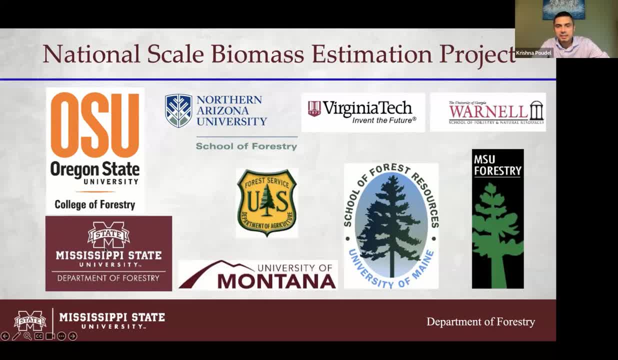 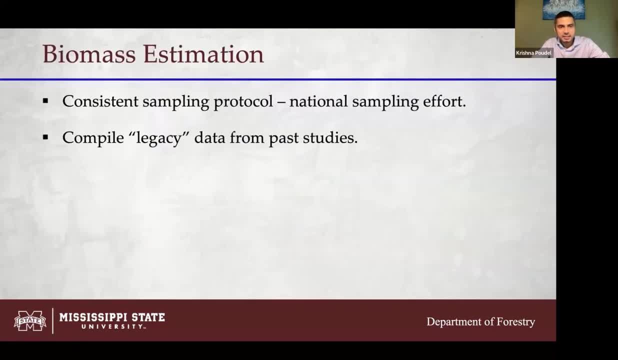 and then when I came to Mississippi State University, I continued that collaboration and other universities were also involved, And what we did is we developed a consistent sampling protocol for the national sampling effort and also compiled legacy data from past studies. So with that data- new and existing previously published data- we evaluated. 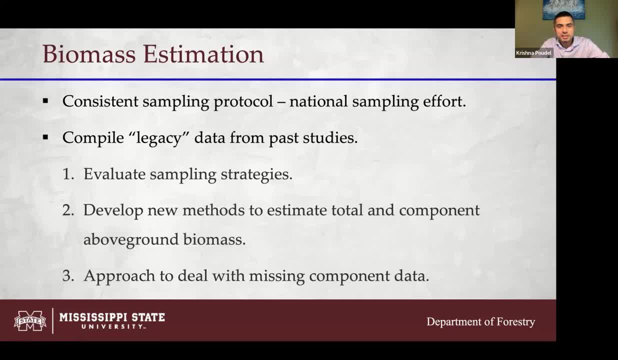 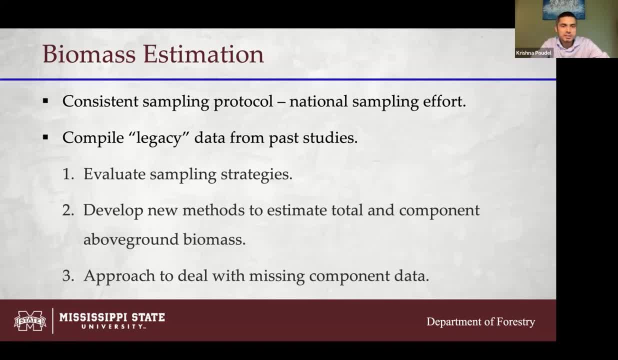 of above-ground biomass. Still, we did not do below-ground biomass, but this was for the above-ground biomass and we also looked at different approaches to deal with missing component. For example, in historical data there were some studies where people looked at 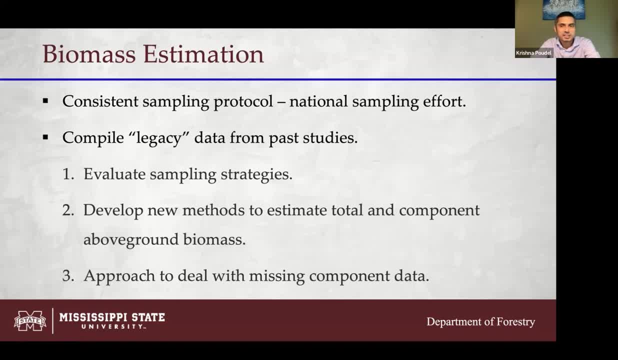 total biomass and just the steamwood biomass. They left the bark biomass. So how to account for the missing component, missing bark component. So different approaches were tested, some imputation methods, and the result of this is there will be new equations and methods. 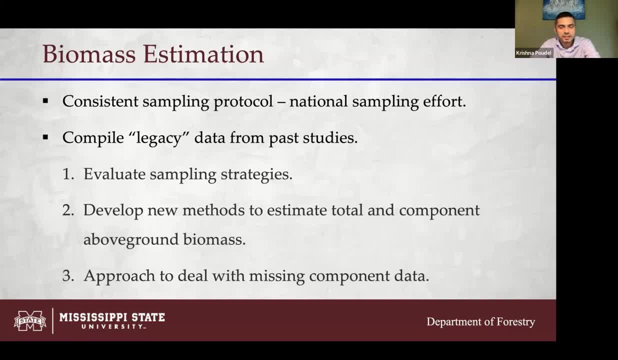 that we will be using in the US for official greenhouse gas inventory reporting to the UN, starting, hopefully, end of this year. So so far what I talked about is measurement of biomass and partly the estimation. but now let's. 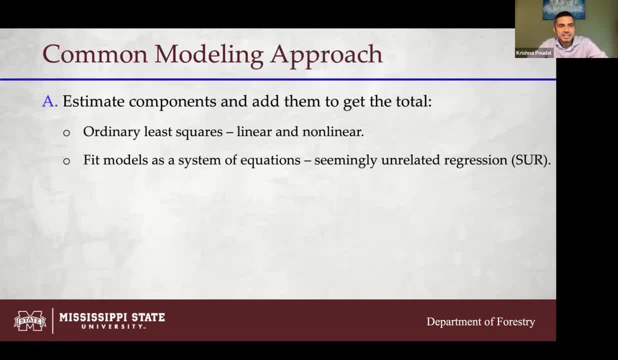 focus on biomass estimation. So let's say that we have the data where we have, let's say, we did some destructive sampling and we obtained the data for total above-ground biomass and different components. And now, because biomass measurement is destructive, so if we want to estimate, or if 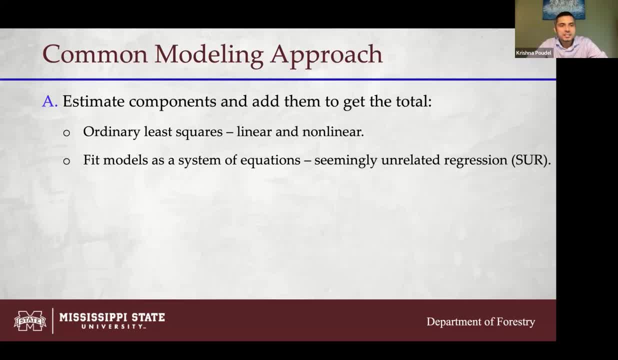 we want to know how much biomass is in the biomass. we need to know how much biomass is in the biomass. If we wanted to measure, then we need to harvest all the trees, but we don't want to do that right. So that's why we need to look at the methods that can help us without help us in. 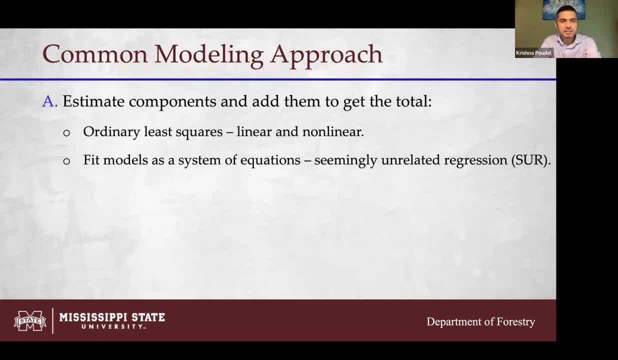 getting, getting or estimating the biomass without having to destructively sample trees. So there are two common approaches. The first approach is estimate the components and add them together to get the total. A common method is to estimate the components and add them together to get the total. 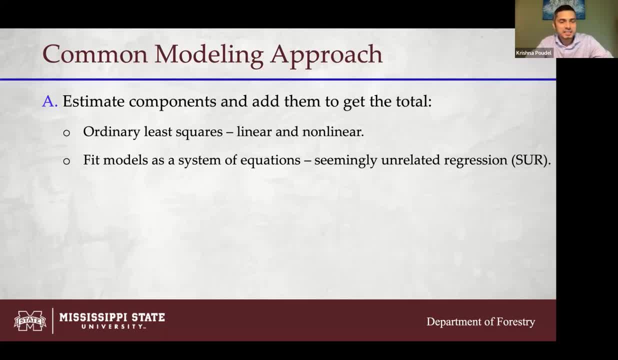 A common method is to estimate the components and add them together to get the total. A common method is to estimate the components and add them together to get the total. A common method we use for that is: we can use linear least square regression or ordinary least square regression. It can be. 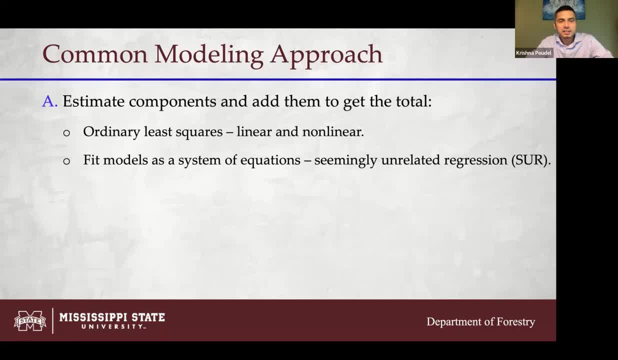 linear or non-linear, and also we can fit model as a system of equation using seemingly unrelated regression. That's a very common practice. And the second approach is first estimate the total and then distribute that into different components. In this case we use some kind of generalized 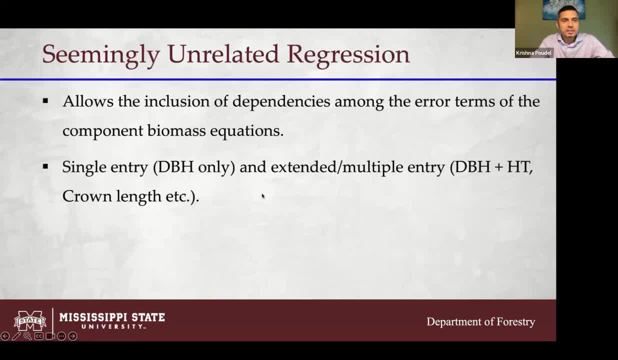 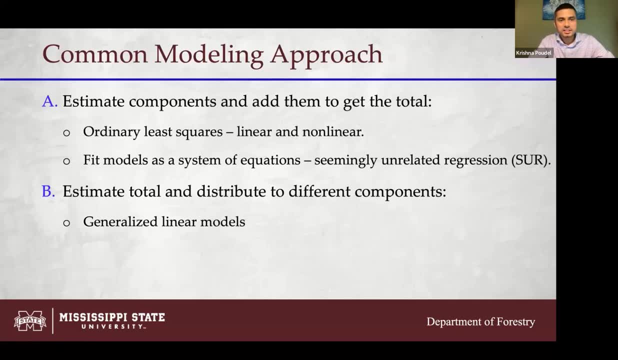 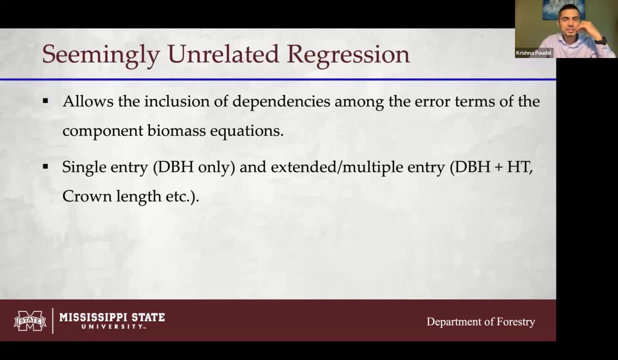 linear models And so ordinary least square, which is, you know, for example, simple linear regression. we can use ordinary least square estimation technique And when we have multiple equations, then we have, because we will be using the same data set for fitting multiple equations. 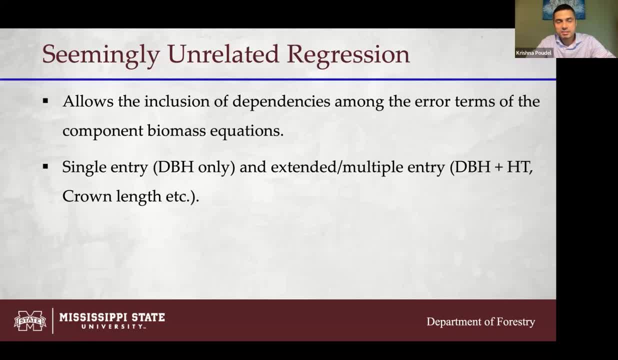 that means we need to take into account the error structure. So using the seemingly unrelated regression, it allows the inclusion of dependencies among the error, because we have component equation, and then the errors. they can be correlated. So we can use seemingly unrelated regression to address that, And they can. 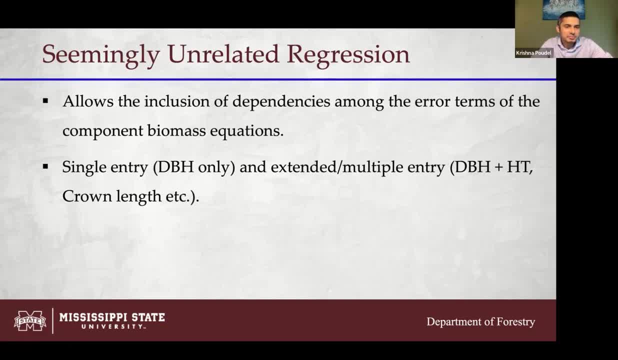 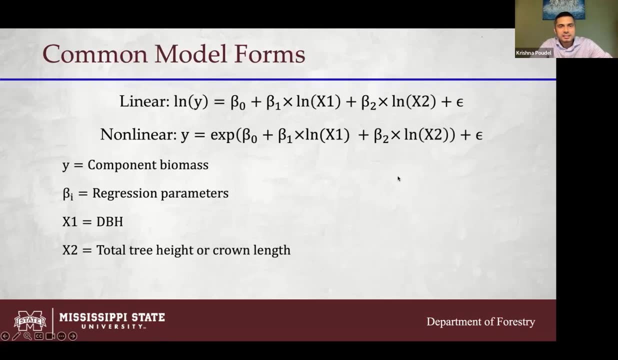 be, or commonly they have been. there have been some single entry or deviates only and extended meaning multiple entry deviates and height or crown length and other predicted values. And there are different model forms people have tried but most common is in linear Usually. 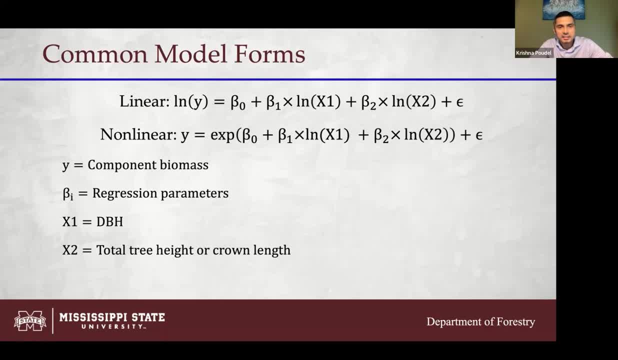 the biomass models are fitted in log scale And so ln, y, so that's the natural log of component biomass, And x1 and x2, we have independent variables. x1 usually deviates and x2 can be any other predictor, potential predictor variable for us. So that's the natural log of component. 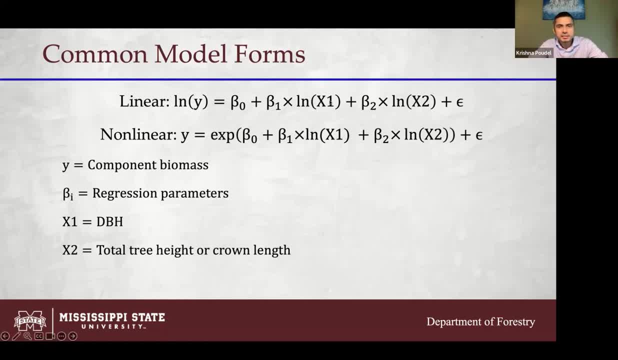 for biomass And we can also fit this equation as a non-linear equation like this: If we take log on both side of this equation, then it would become linear And there is also another power model. people use So many different type of equation, equation form used, but 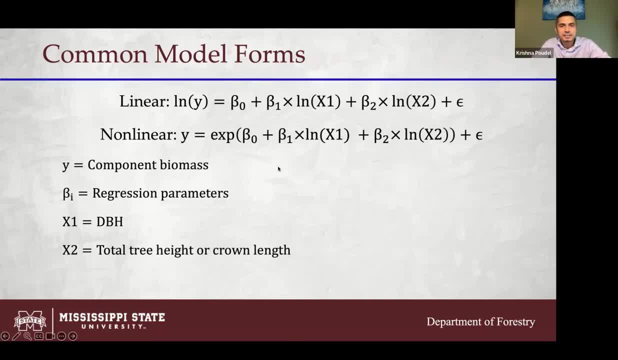 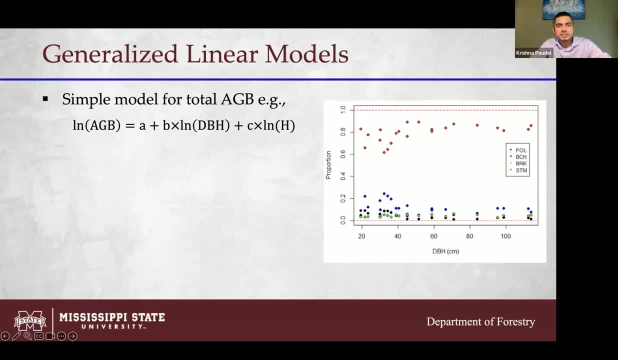 these models act better when we fit that as a linear modeling, log scale And for the generalized model. if we so, this one would be aggregation approach, And for the disaggregation approach we can fit a simple linear, not simple linear, but simple or just a. 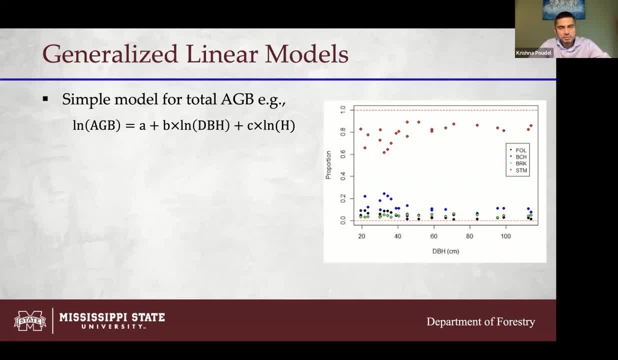 linear model to get the above ground biomass, total above ground biomass, And then we can use different generalized models to predict component proportions. For example, beta regression is one, Dirichlet regression is another one, And there are other options as well. 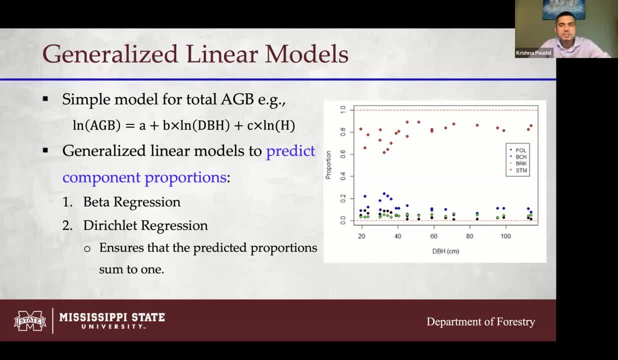 but I talked about this because these are the models that I have used. So basically, get the total and then get the proportion. what percent should be in each component? Looks like there's some chat, Okay, Okay. So, and the differences between beta and Dirichlet regression is. 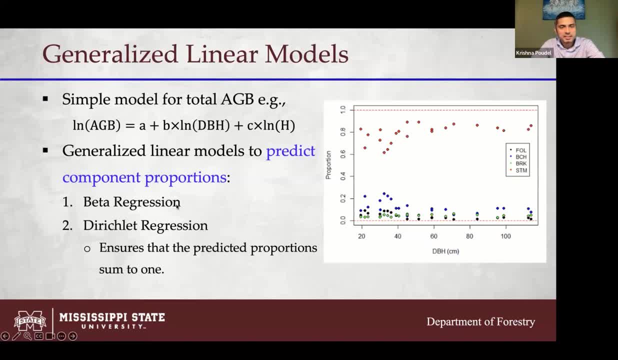 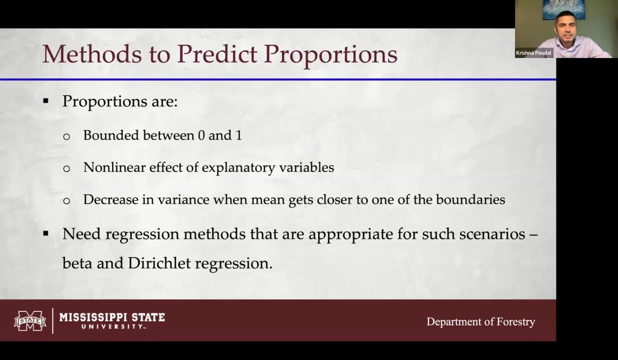 beta we fit equations independently. So, for example, if we have four components, those components will be independent of each other, But Dirichlet it fits the equations simultaneously so that it behaves well, or it behaves better than beta regression. And so why do we care about these instead of using ordinary least square? why do we care about? 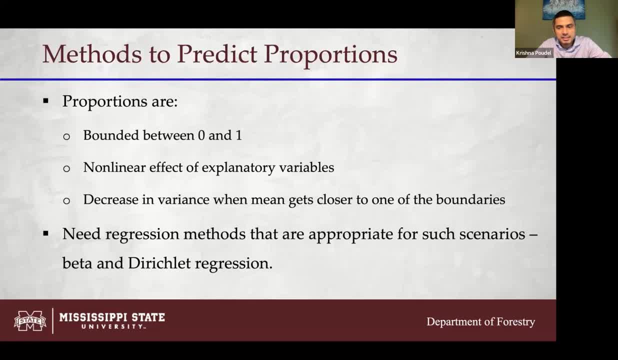 this different type of regression models, generalized linear models, because if we want to predict the proportion, then they have different properties. for example, they are bounded between zero and one. when we fit actual biomass, for example, in terms of kilograms, then the values would be between zero and however many kilograms the biomass is. but if you, if we want to predict the percentage of 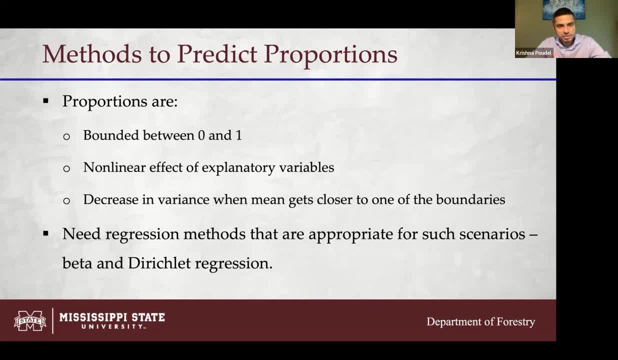 biomass in each component. then they will be bounded between zero and one, zero percent and hundred percent. hundred percent will be one and for that the effect of explanatory variables, for example dvs height, that can be non-linear and the variance decreases when mean gets closer to one of. 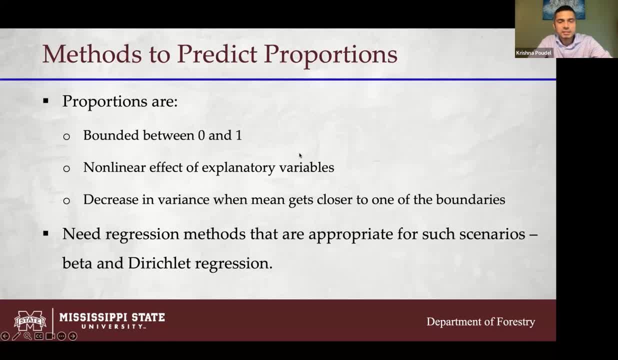 the boundaries. so when mean is close to zero or one, then the variance gets, variance decreases. so that means we need regression models that have capabilities to address those challenges and beta and Dirichlet regression- they they have that capacity, so that's why we can use them for predicting proportions. and briefly about the 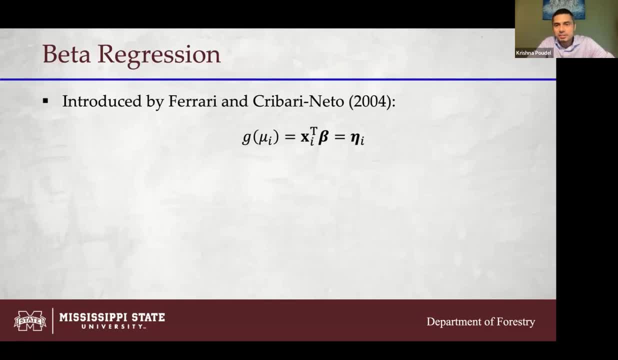 beta regression. it was introduced by Ferrari and Krivary Neto in 2004 and I'm not sure how much experience you all- everyone- has in fitting generalized linear models. but in generalized linear models we have a link function and then we have the matrix of dependent variable. 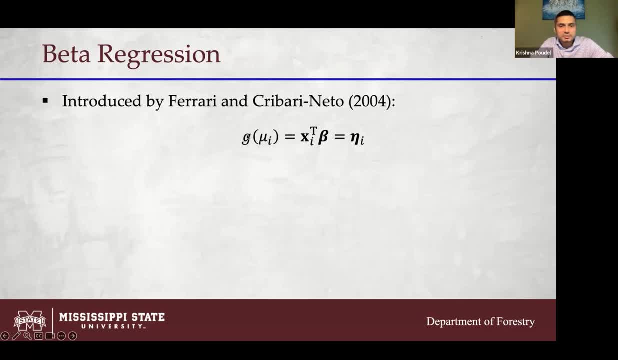 and the regression coefficients, and this is related to mean through that link function. so, like I said, this g is the link function and in beta regression we can use different kind of link function. and what is the effect of that is what kind of link function we use determines how the 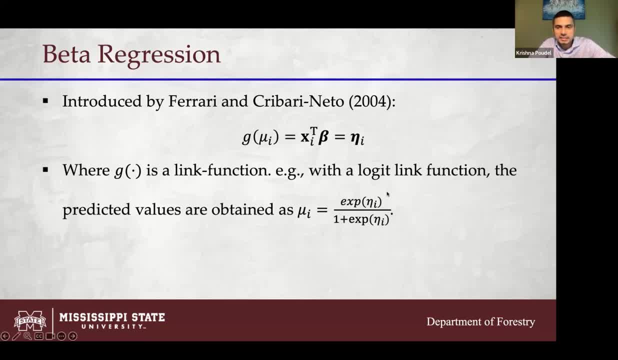 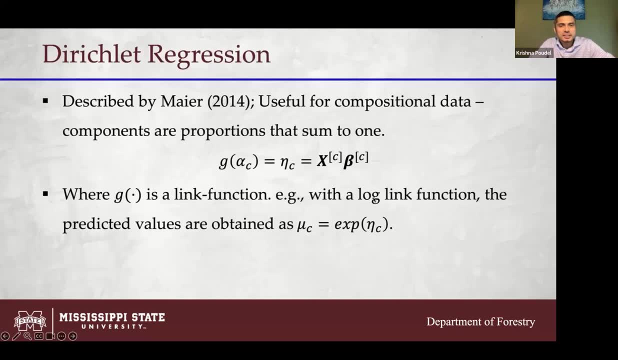 prediction will be made. so, for example, if we are using logit link function, then mean or estimated mean will be calculated this way and Dirichlet regression is based on the Dirichlet distribution, which is the multivariate. in beta regression we have one component, but in 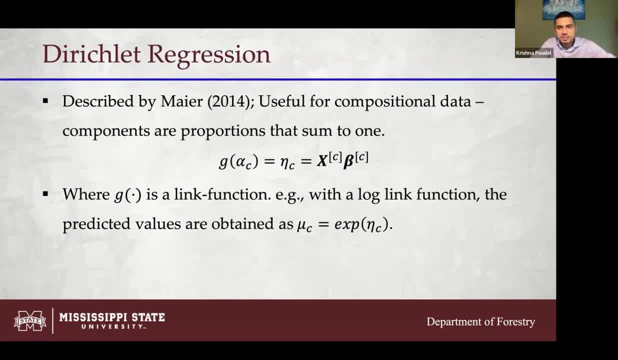 Dirichlet regression or Dirichlet distribution. we have multiple components, so it's a multivariate generalization of the beta regression or beta distribution and it is useful for compositional data. compositional data is if we have different parts and then they add to one, then we have a. 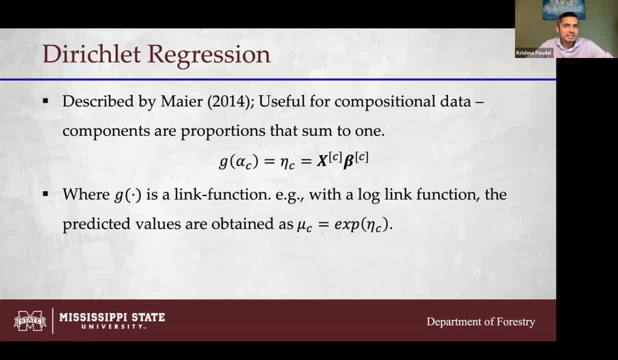 compositional data, for example biomass proportion. we have, let's say we have four components: stream wood, steam, bark, foliates and branches, and then if we calc, if we use the proportion or percentage, then they add to one. so so in that case the Dirichlet regression is useful and one advantage of one better property of the Dirichlet. 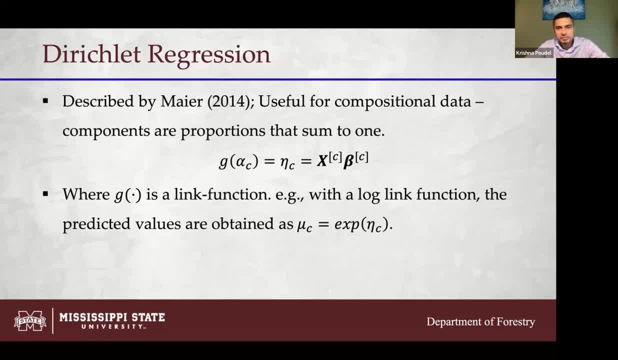 regression is when we fit different components, components simultaneously, when we model them simultaneously, meaning together, then the sum of the predicted values for different proportion will be one and also same. as in beta regression, we can use different type of link function and that determines, uh, how we calculate the predicted value. 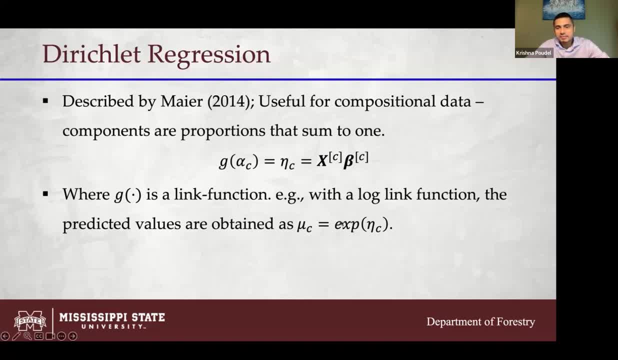 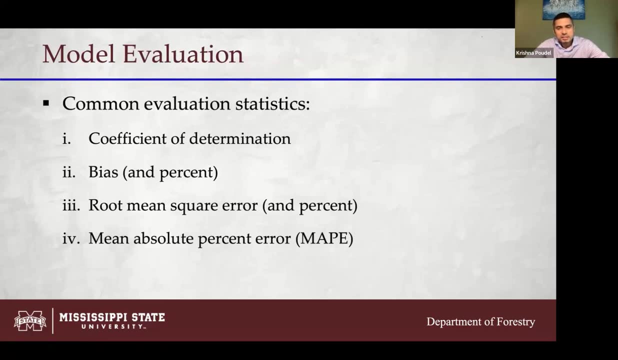 and if, for example, if we are using log link function, then we would calculate by just exponentiating the um Eta. it's called Eta, so that's the linear predictor. so basically, once you measure the measure biomass, then we fit regression models. there are different types of regression models available and once we fill the model we need to evaluate how good they. 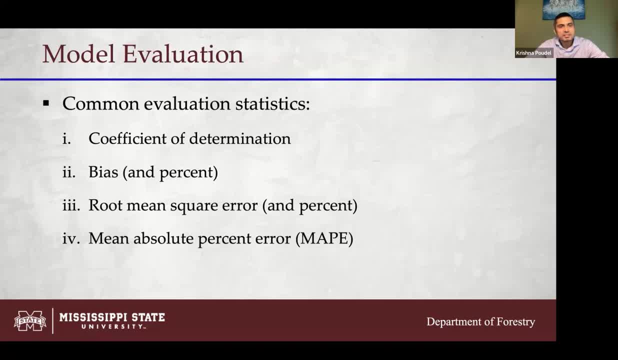 are and common evaluation statistics. we use coefficient of determination R square, which tells us how much of the variation in a dependent variable is explained by the independent variables. bias, or the mean difference in observed value and the predicted value, and also percentage and root mean square. error, which combines both bias and the variance. 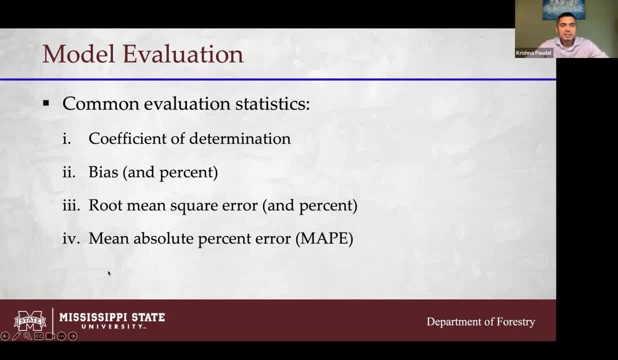 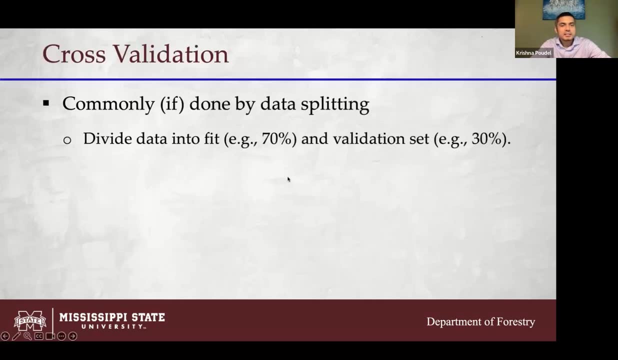 and also the percentage of root mean square error. and then we look at the mean absolute percent error map. so mean absolute percent error and that's also another commonly used statistic in evaluating the model model fit. and then model validation is. I would say it's not that common because, you know, because the biomass data is usually not 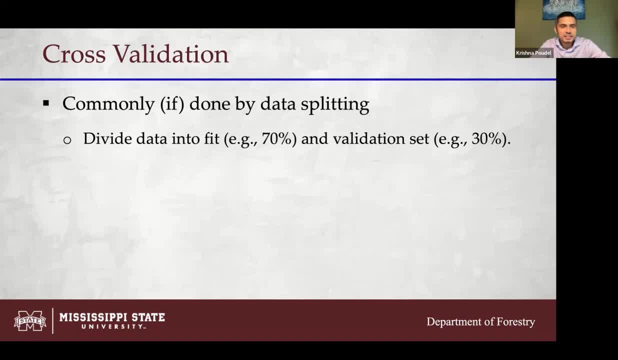 that large. so, but if it is done, usually it is done by data splitting, sometimes using leave one out, um, so, for example, you leave one tree outside of the data and then fit model using the remaining trees and then apply the fitted model to that one tree and then calculate the evaluation statistic. 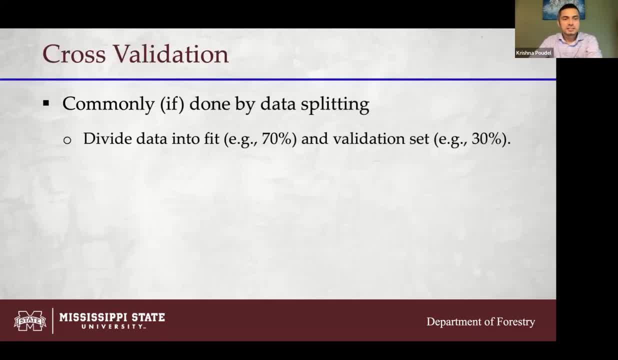 square and so on. and in data splitting, for example, we can divide data into 70 percent for model feeding data and validation data, set for 30, using 30 percent for model validation. so basically, we use feeding data to get the coefficient of the model and then apply those. 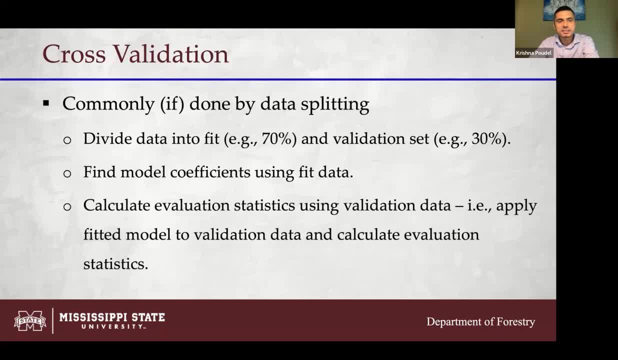 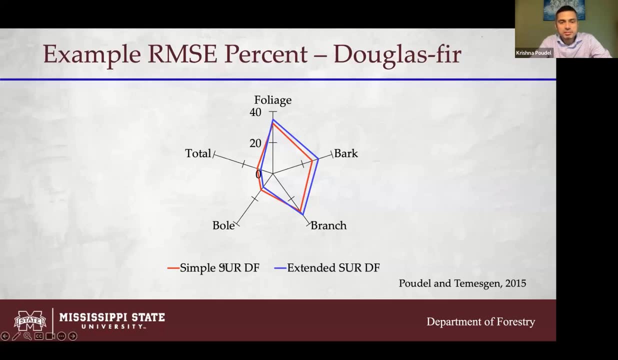 coefficient into validation data and calculate the evaluation statistic and at the end we average those evaluation statistics to get one value for a given model. so here is some example of root mean square error percent using a simple sur meaning dbs, based, as you are, seemingly unrelated regression and extended, uh, seemingly unrelated regression for douglas, for trees, which. 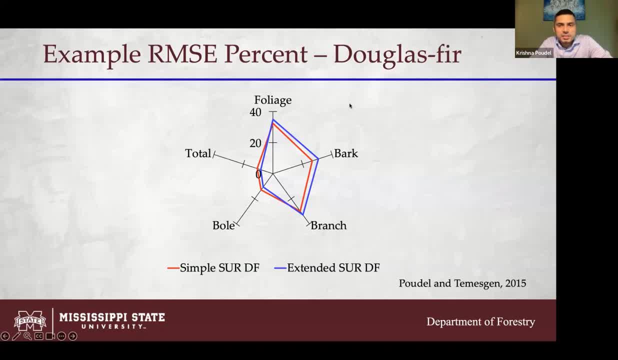 is, like i said, uh, a common tree species in pacific northwest, in the united in the us, and uh. so you can see these are percentages. so we have higher percentage of error in foliates, but because foliates is a smaller amount compared to the ball biomass or the stingwood biomass, 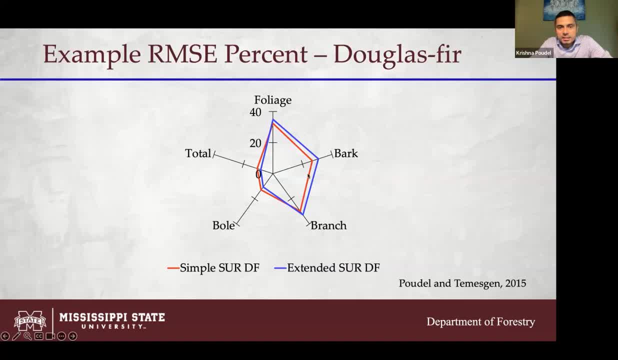 so in terms of absolute unit, this will be smaller. so the blue is the extended sur and the red is the simple, as you are. so if we look at the total, by using extended meaning adding height instead of just using dbh as the predictor of biomass- we can. 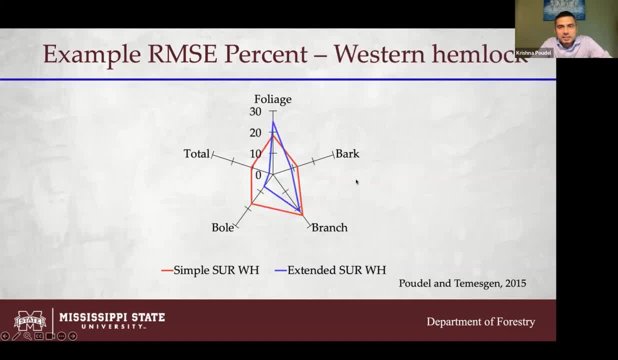 reduce some error. and then this is for another species, western amalek, another common species in pacific north, specific northwest, and we see a similar trend. so here, if the area covered within this polygon is a small length, that will be a better, better method. ideally, i would have liked. 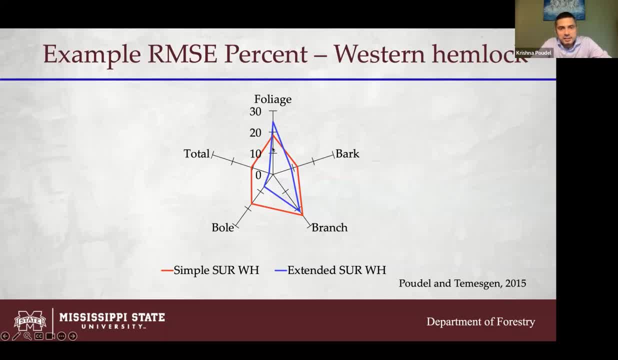 this to be inside here as well. so that way i could say the extended or extended sur is giving smaller error for all the components. but here, uh, extended is actually because this was fit as a system. so overall for the total it is way smaller than the dbh only model. 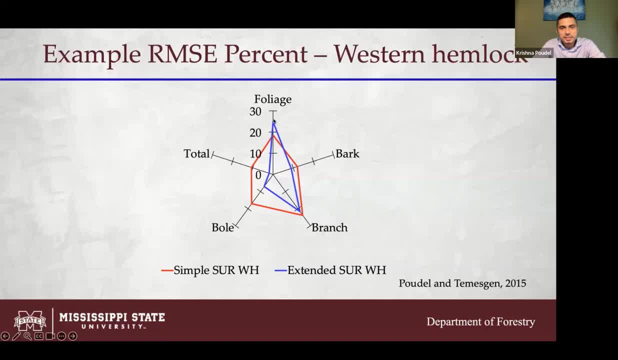 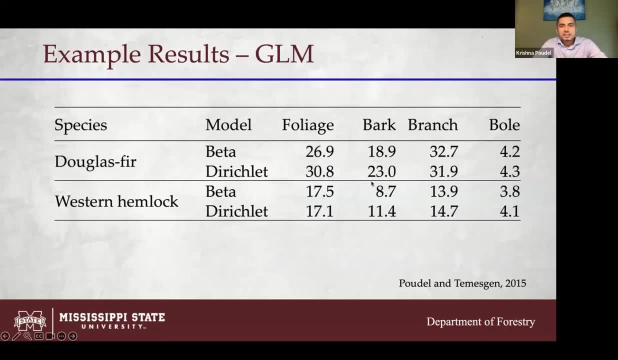 but uh, for some component, especially for foliates, the error was higher than uh, using dbh only model and uh, this is uh same similar result, uh, but in table, uh, and using the generalized linear model beta, and it is the regression now. so here we see that uh. so for douglas, for. 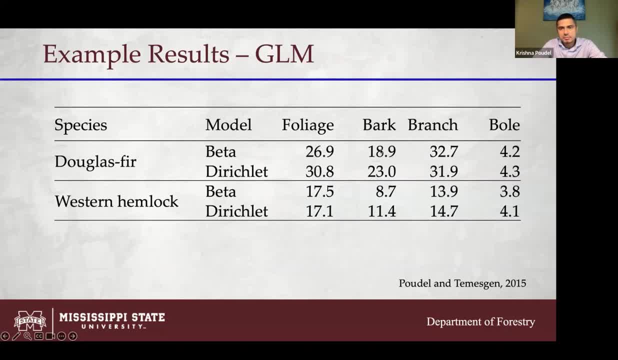 beta is doing good. uh for foliates and bark biomass, uh, not so for the branch biomass, and once again for the ball biomass and uh for western hemlock. dd slay is doing better here. not so much here, not so much in other component. so basically, not one model was good for all component. 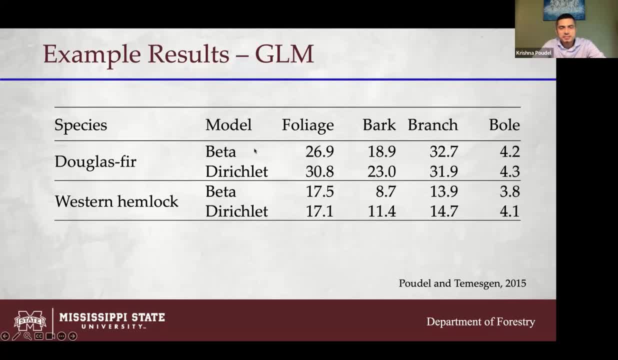 but looking at the properties, beta regression provides four different proportions and those proportions may not add to one. but dd slave provides the uh estimated proportion for all components simultaneously and then they would add to one. so that means the it has uh, maybe slightly higher error for some component, but it is uh, it has that. 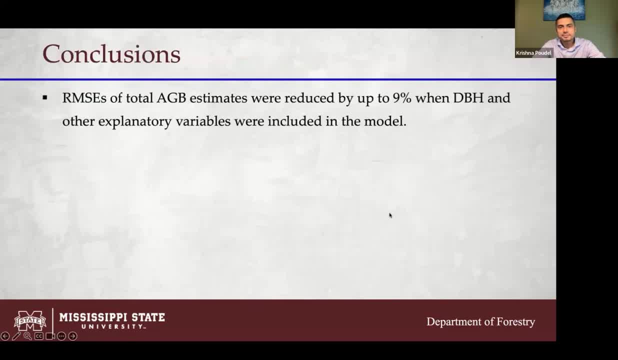 better property of um additivity. so, in conclusion, root mean square error for total above ground biomass estimates were reduced by up to nine percent. when gbs and other explanatory variables were included in the model Methods to predict proportion, they were unbiased and produced smaller root-mini-square error compared to the SUR. 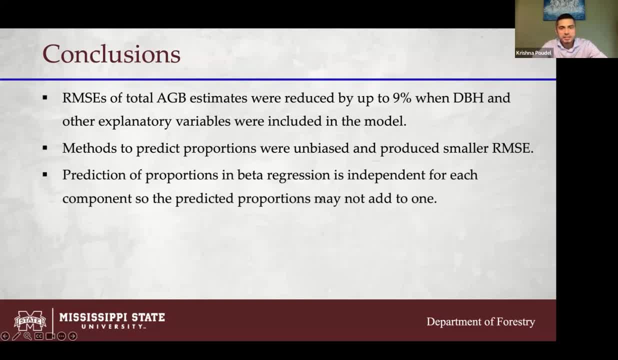 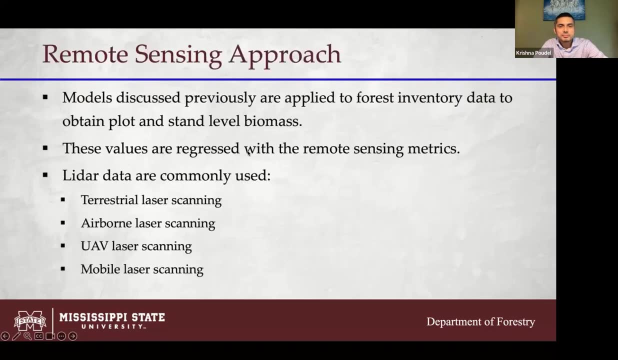 And prediction of proportion in beta regression is independent for each component, which means the predicted proportion may not add to one, but the Dirichlet regression that solves that problem. So the sum of the proportion will be one. And briefly about remote sensing approach. of course remote sensing has gained a lot of attention in the recent, maybe a decade or more than that. 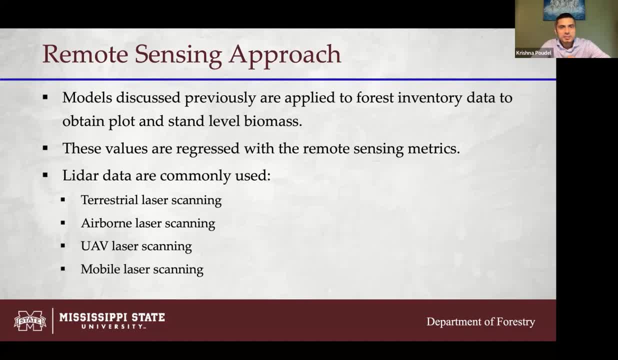 And the application of remote sensing approach in biomass estimation is: first we apply the models that we just discussed and to the inventory data and get the plot level or stand level biomass, And those values are then rigorous, And then we test using remote sensing metrics. 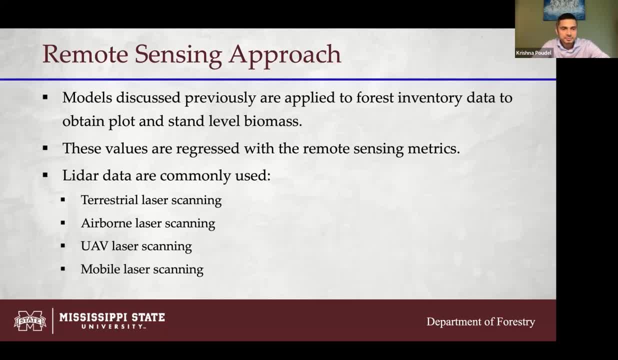 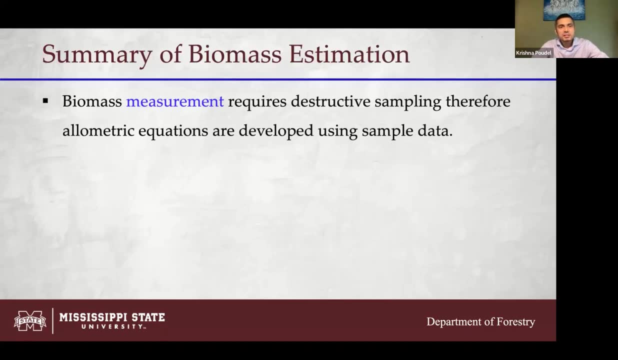 LiDAR is commonly used in the US, For example, terrestrial laser scanning, airborne UAV laser scanning, mobile laser scanning, So there are different types of LiDAR data that we can use. So to summarize, biomass estimation measurement, like I said at the beginning, there is one component, which is measurement.